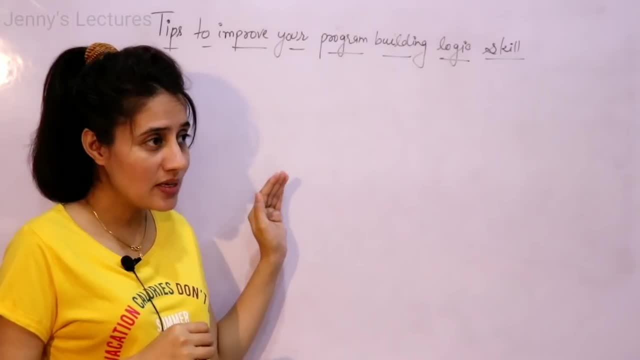 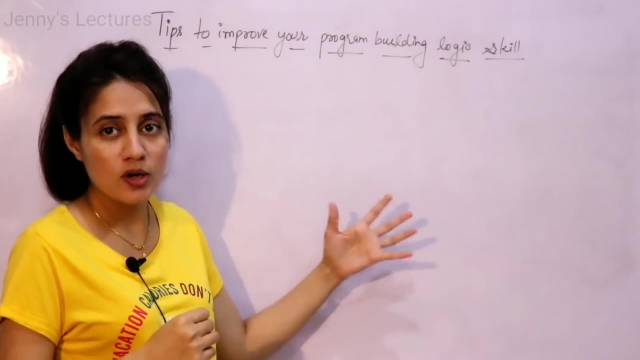 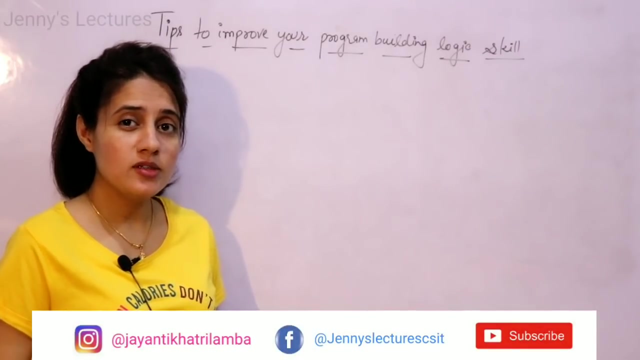 So you can follow these steps means the mistakes I am going to discuss that many students do, and plus the solutions for those mistakes means what you should do to improve your Program. you know building logic skills right? So many students are facing this kind of difficulty. 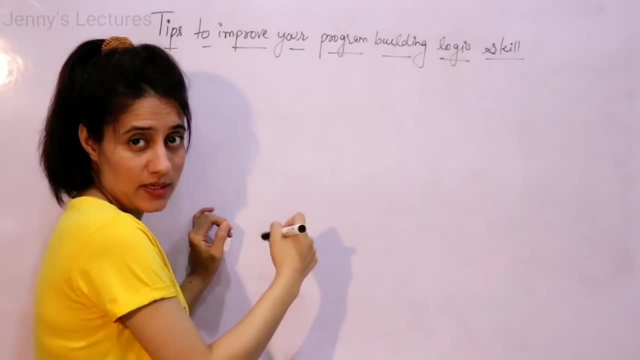 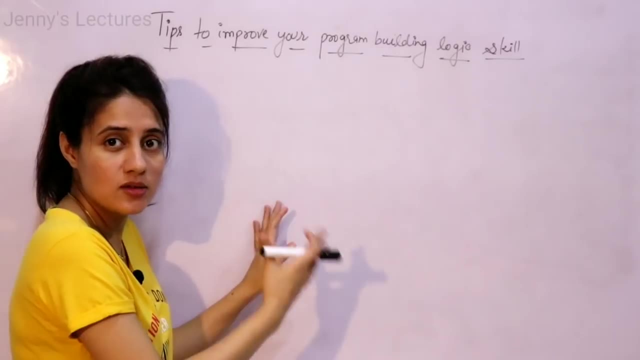 Like. suppose I am here describing any program or any code. in that case you are able to understand that code right One by one. I have already discussed many times the code or the logic and I have dried in that program on the board. 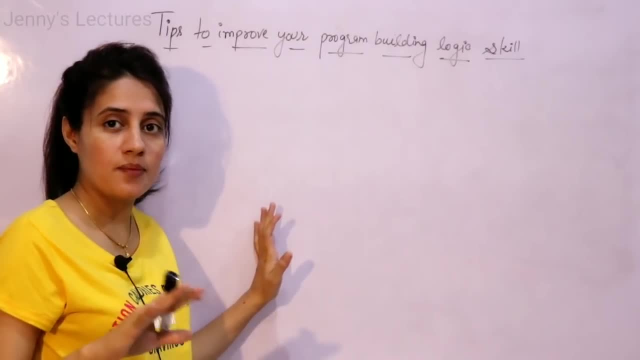 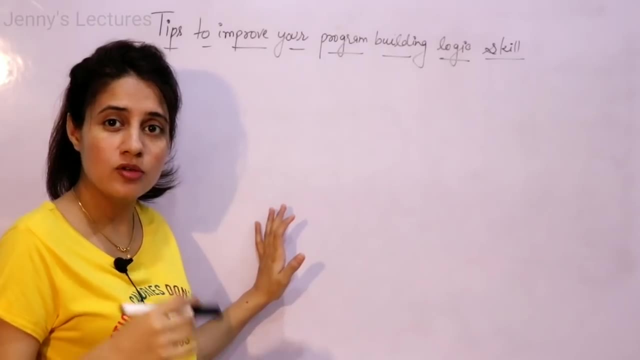 Maybe at that time you are able to get that logic and you think that, yeah, I got it. But when it comes to you means you sit down and you write down the code, you start writing the code, you just go blank, right. 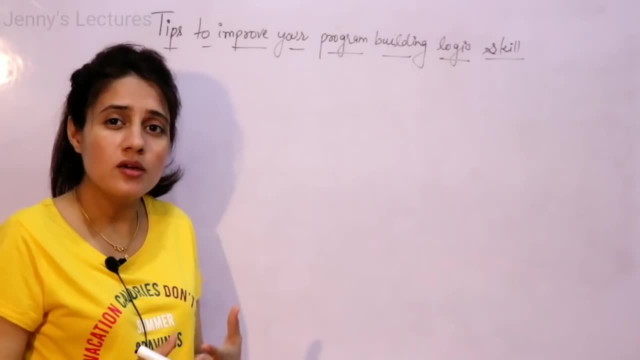 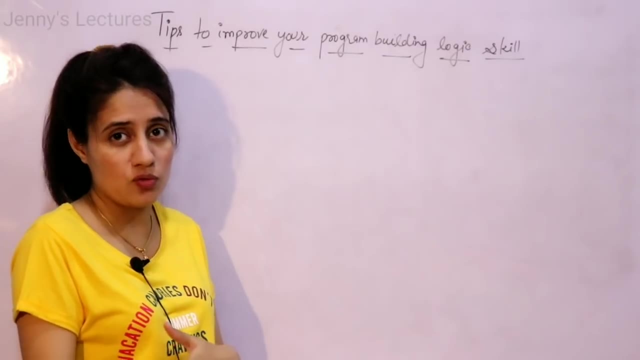 Means you can understand the code but you are not able to think at your own right. Or sometimes, maybe some students are not able to even understand the code and they are not able to write down the code right. So these kind of difficulties you must be facing, fine. 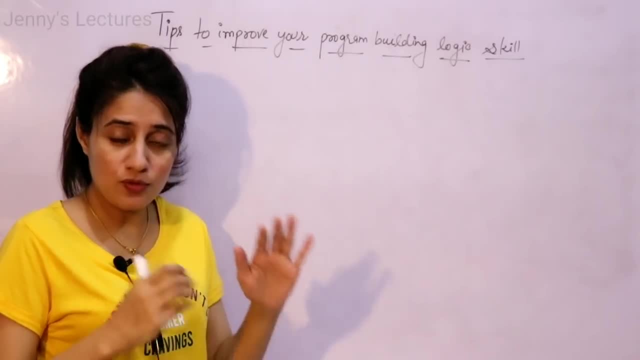 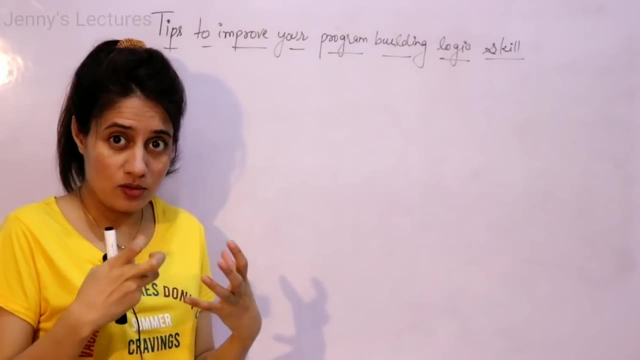 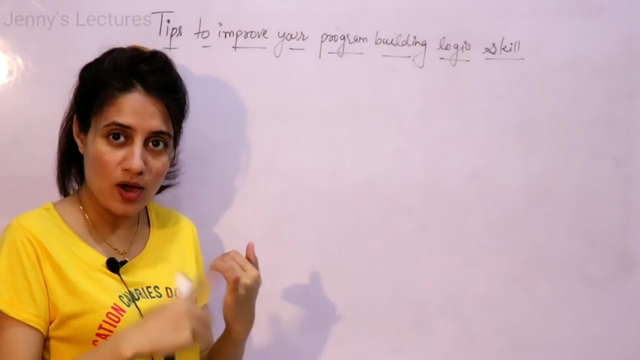 So the very first step is what? If you really want to, If you really want to be good in programming, if you really want to, you know, improve your building, the you know, programming logic skills, then first of all you have to be patient and you have to practice. 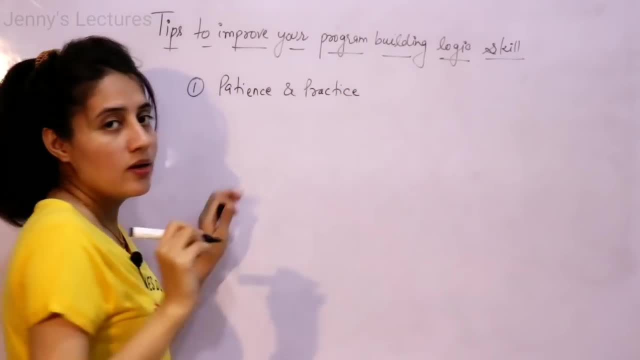 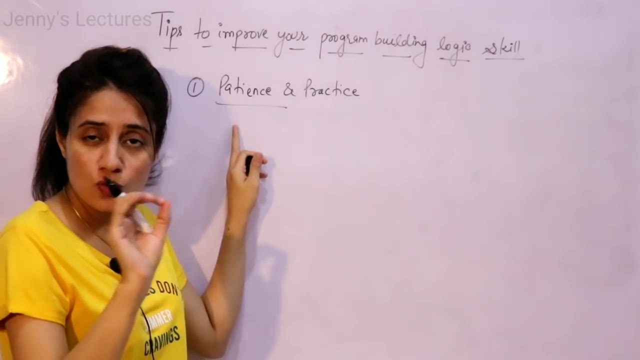 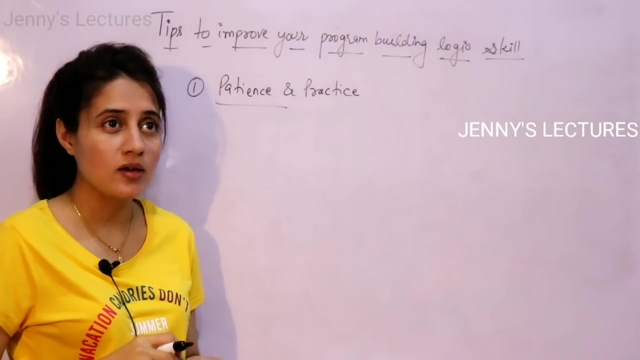 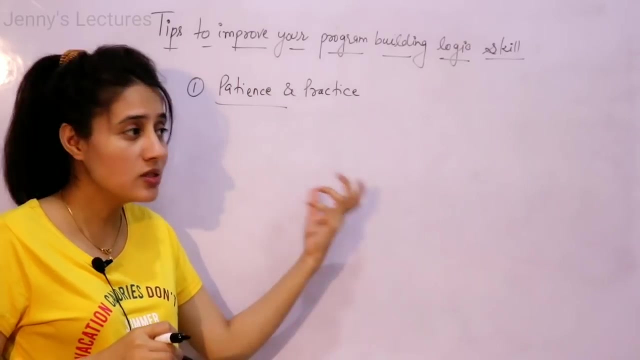 The very first step is what? Keep patience and practice. This is very important Here. patience means don't give up. It's not like that If your colleague or your classmate is, You are not able to think the logic, and you are here, you are not able to think the logic. even you have tried 10 problems, 15 problems or 20 problems, but still you are not able to think the logic. then what you will think? 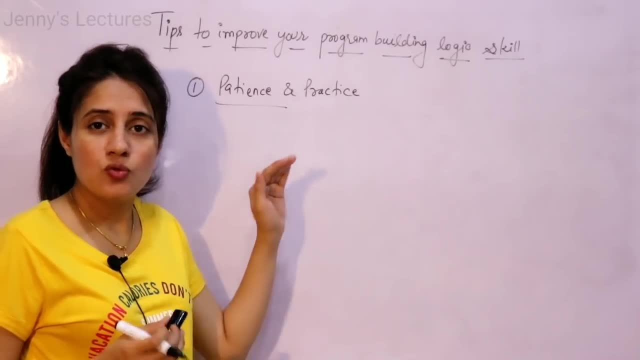 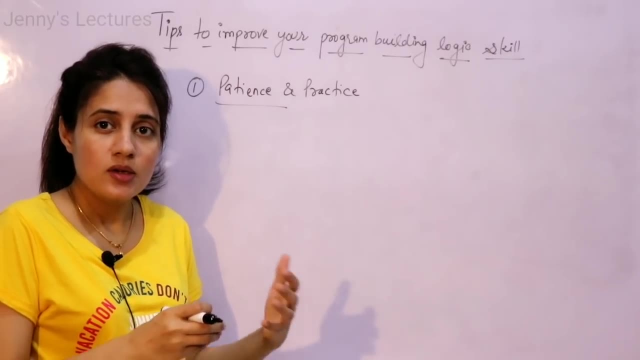 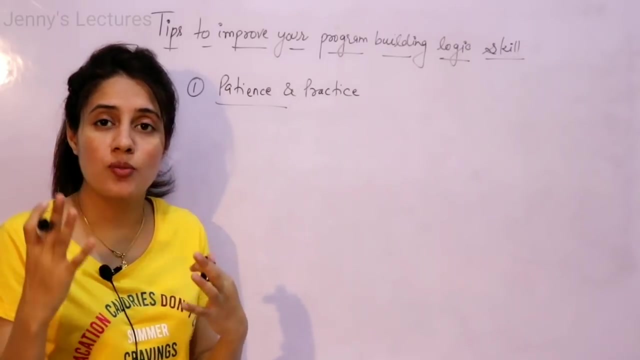 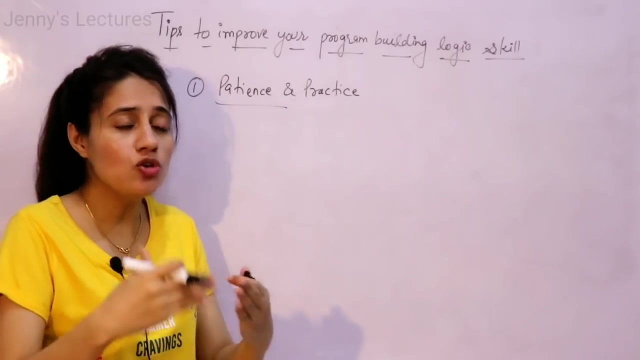 Please don't do this. Don't give up. first of all, maybe after solving 50 problems or 100 problems, definitely a time will come that when you will see a problem automatically, the logic will come into your mind. Maybe 20% logic, 30%, 50%, not exact, but to some extent you'll be able to think about the solution of the problem. 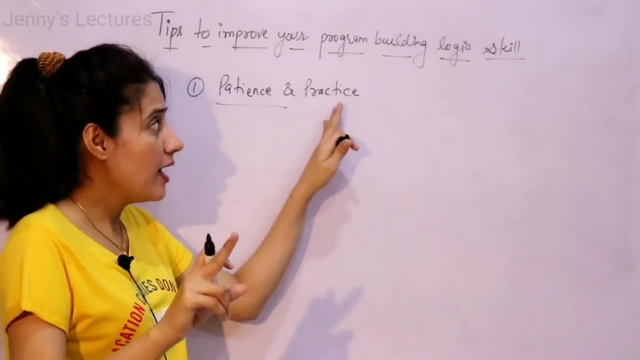 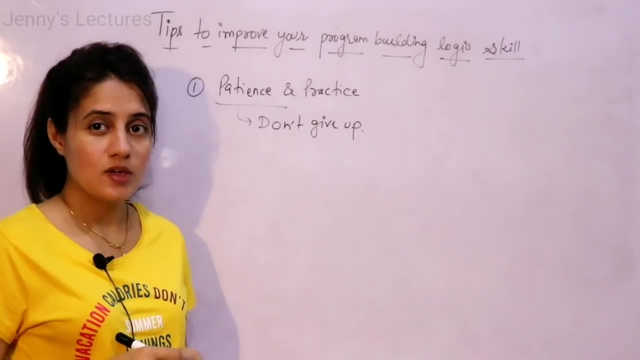 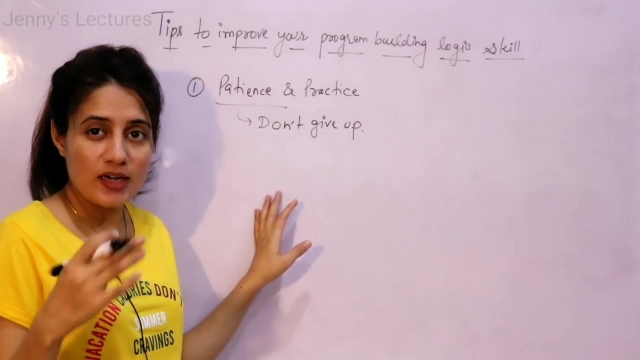 Right? So you have to keep patience and you have to practice very hard, Right? See, there is no shortcut for success. So if you have that patience, then only this video would be helpful to you, Right? because ultimately, maybe, 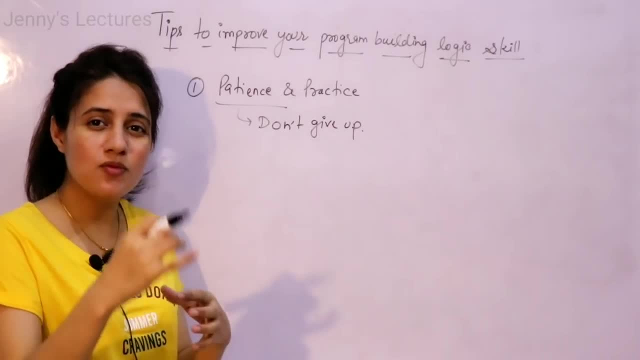 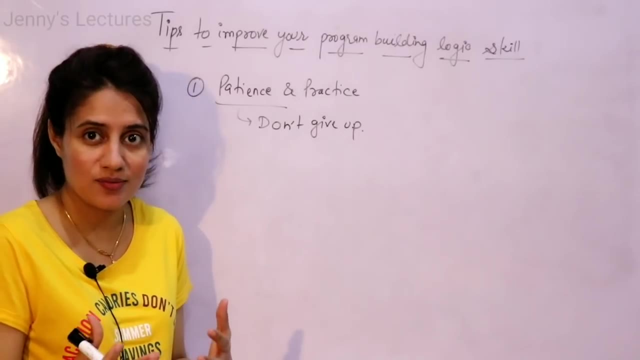 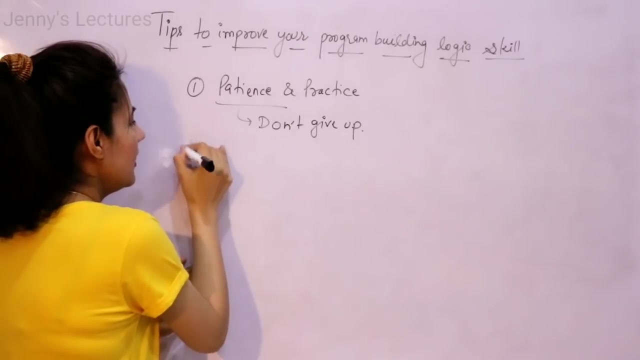 After practicing for for 15 days or maximum for 30 days. if you practice regularly, definitely you will see the improvement. you will feel the improvement in yourself, right? you are able to think the logic right, so don't give up. and practice hard, right? secondly, theoretical knowledge is also important. it's not like that. 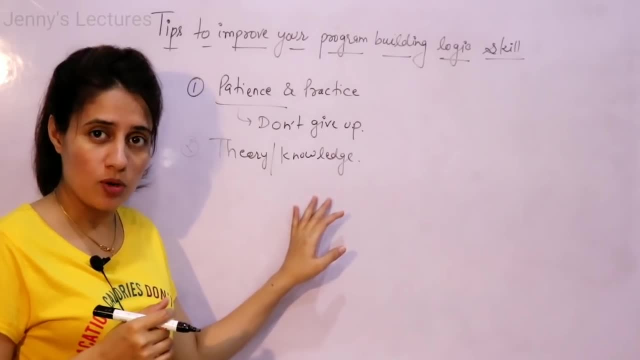 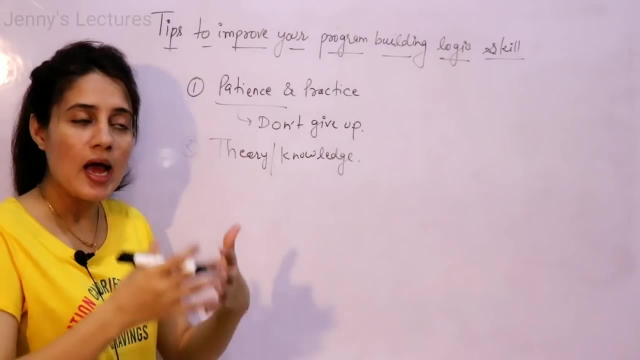 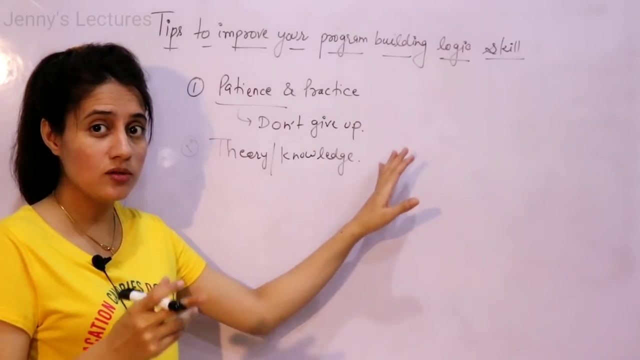 i'm not going to read the concept, i'm just going to practice the problems right, because practical is more important than theoretical knowledge. no, first of all read the concept thoroughly, have the knowledge of that concept, then practice right. but see before implementation or before solving the problem. only theoretical knowledge is you can say it's half complete. 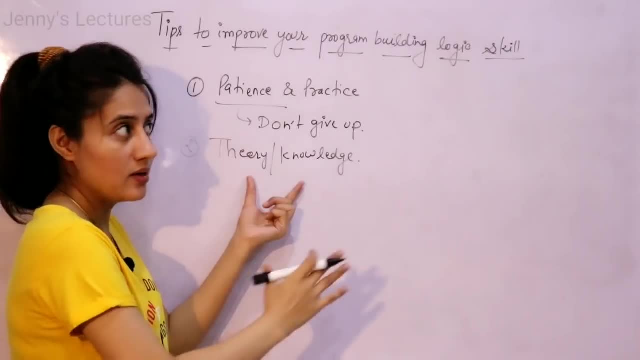 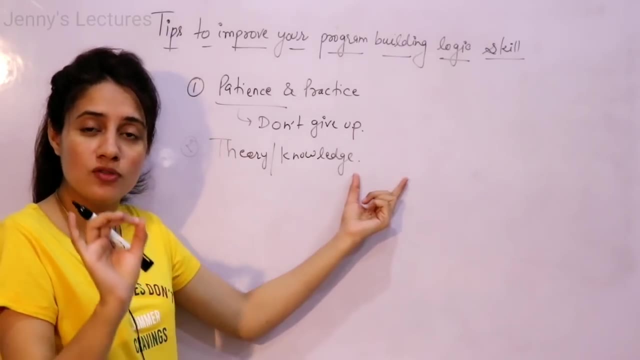 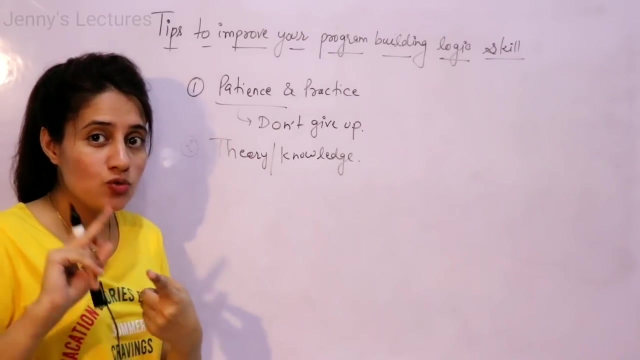 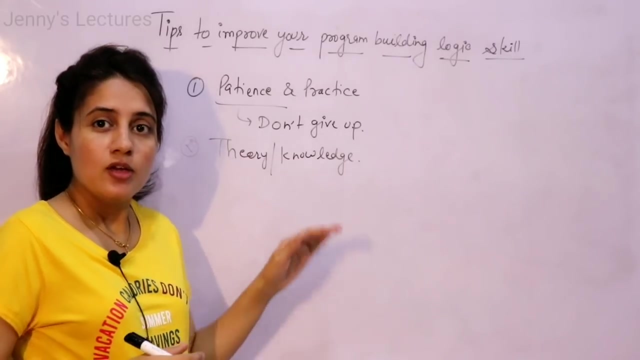 right in case of this, programming concepts, like if you really want to build the programming logic. so theoretical knowledge is also important, plus practice of the questions of those concept is also really very important. right, see, the common mistakes students do is what means generally, when we read the any chapter of a book, fine, we generally read the chapter and 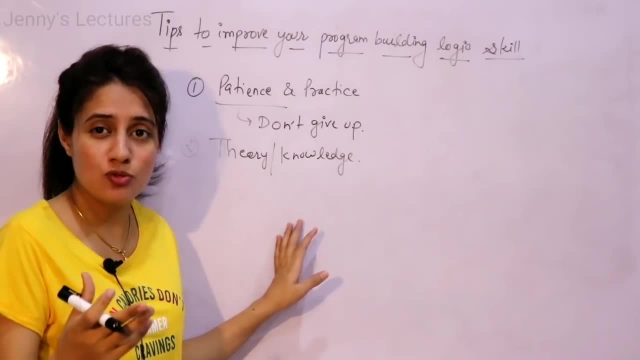 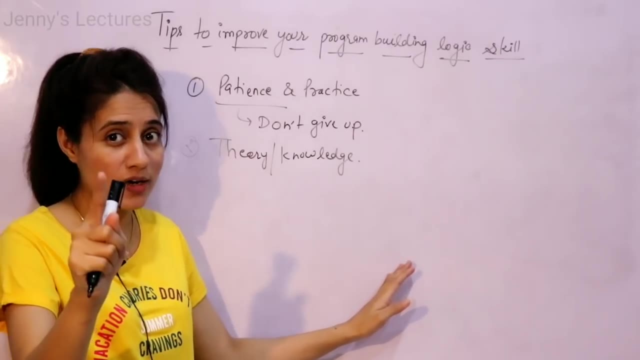 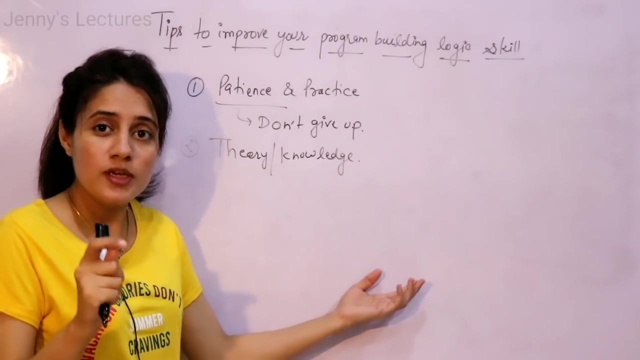 almost 95 percent. 95 can 99 percent students skip the problems or the questions which are given at the end of the chapter. in every book you will find out the problems, but we, we don't bother to see even the problems, right? so please don't do this if you just want to pass out the, pass out the semester. 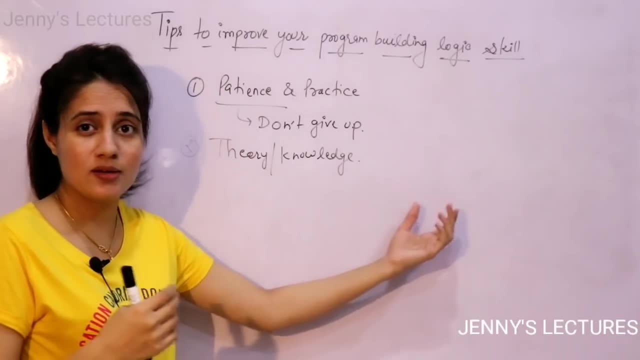 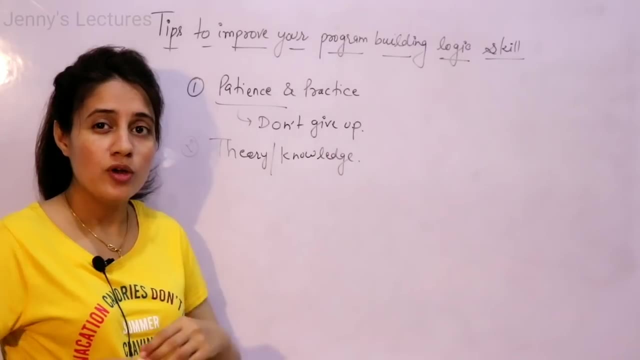 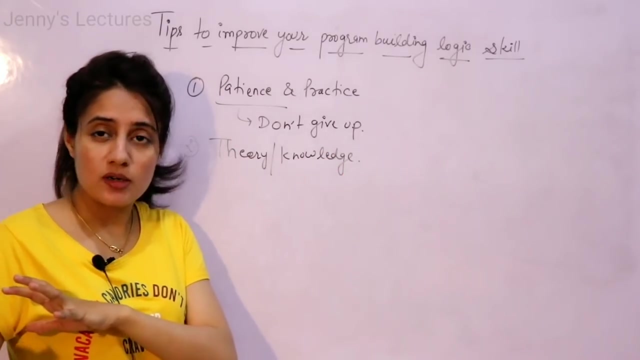 it's fine, just read the chapter and just you know you can ignore those problems. but if you really want to stand apart, if you really want to, you know build the programming logic, or in any case i'm not saying it's for the programming, only for any subject. if you really want to, you know broaden. 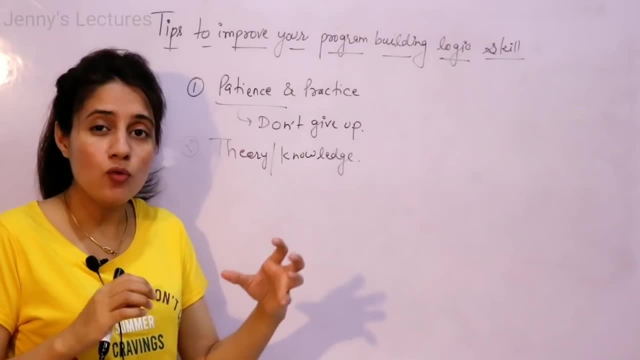 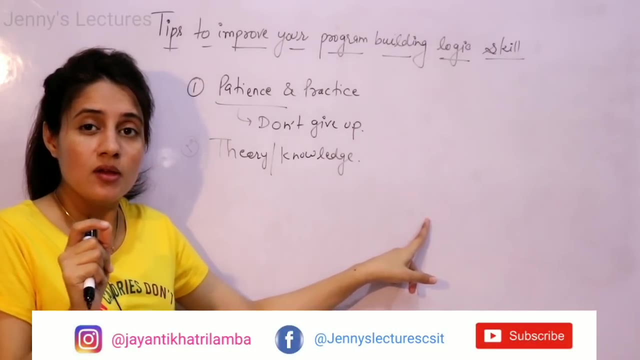 your knowledge about that subject, right, if you really want to, you know, broaden your knowledge about that subject, right, if you really want to, you know, broaden your knowledge about that subject, then you must go to those problems, see, sometimes you see that you have thoroughly read the chapter. 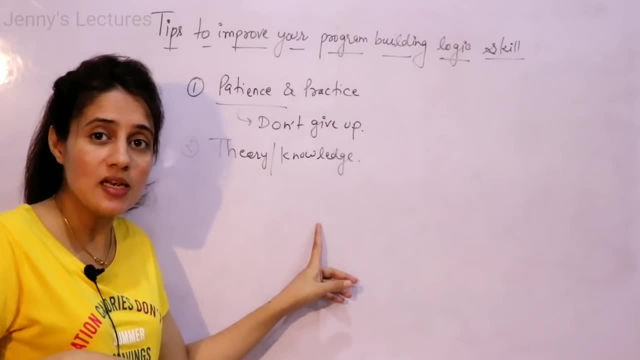 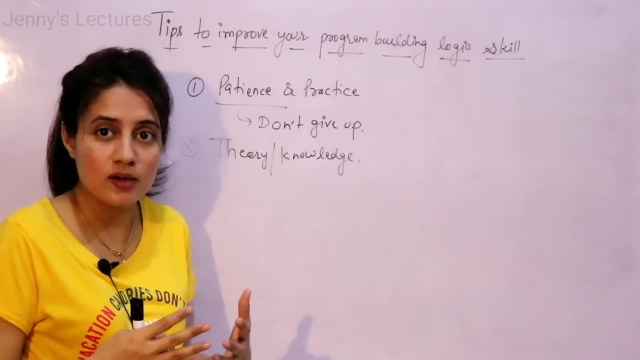 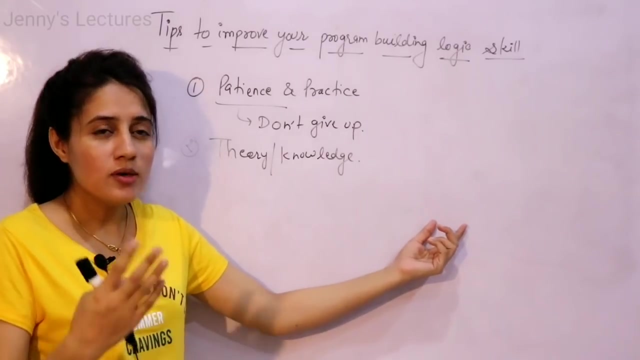 you are very good in that chapter, right. but still some problems are there at the end of the chapter that you are not able to even. you know. understand those problems, right. maybe some problems you can solve, but some problems you are not able to even understand. so these are, some problems are twisted. 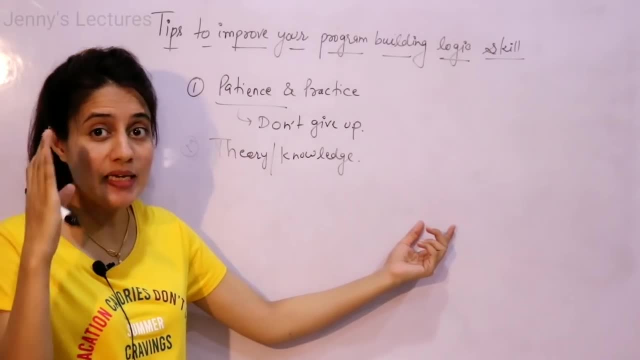 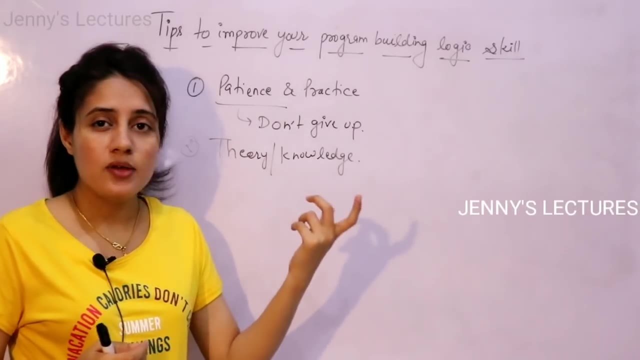 type of problems, so those will increase your understanding of the problem, right? so if you are not able to even understand those problems, right, but still some problems are there at the end of the chapter, thinking capability, right same with like uh suppose, um you are having, obviously you have the you will. 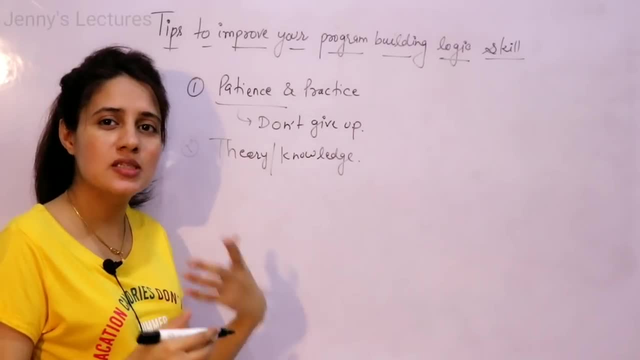 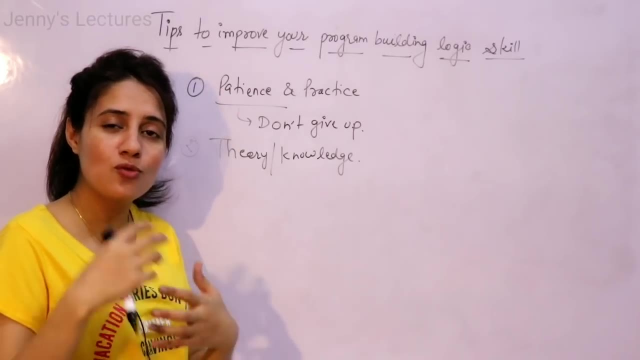 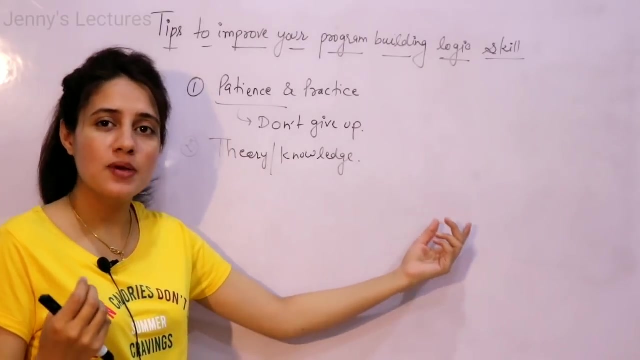 pick any language like c or c plus plus. mostly we will pick c first of all because that is very simple language. if you know how to you know implement the program, or if you have good knowledge of c, then it's not a big deal for you to learn c plus plus- and plus java also right. 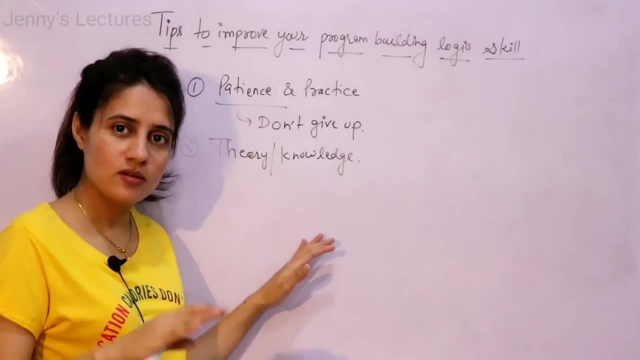 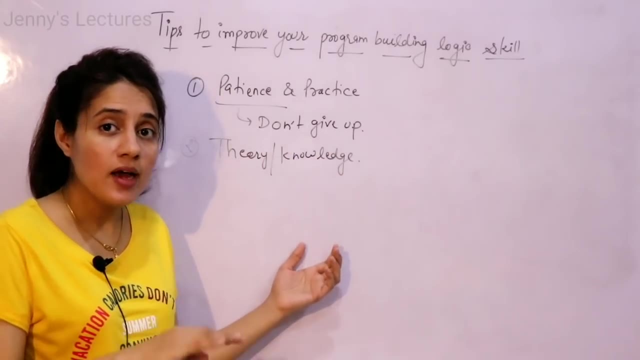 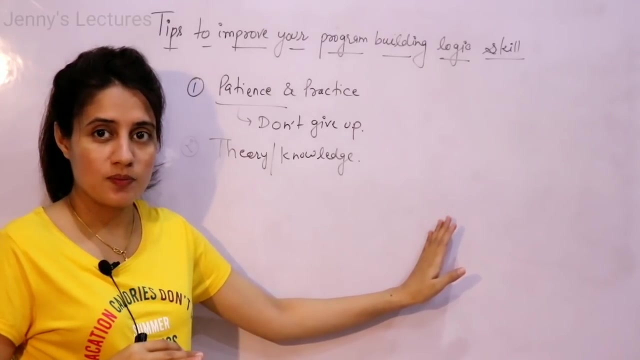 so you can choose first c. if you are a beginner and you want to choose a simple language, so go for c, right, and you read any chapter after that. you must solve the problems at the end of that chapter. we generally skip those problems plus. second thing is: what suppose i am saying? the 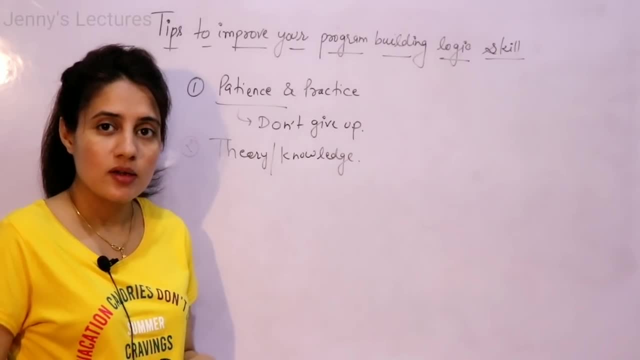 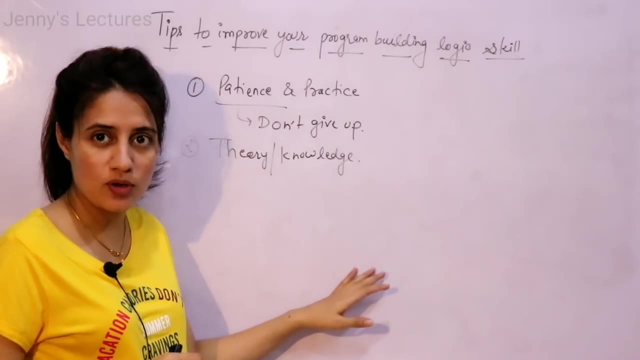 program is what just addition of two numbers right, and when you have any of your colleague done that program or classmate, and you have any of your colleague done that program or classmate done that program or your faculty has done that program, you will think what, yeah, this? 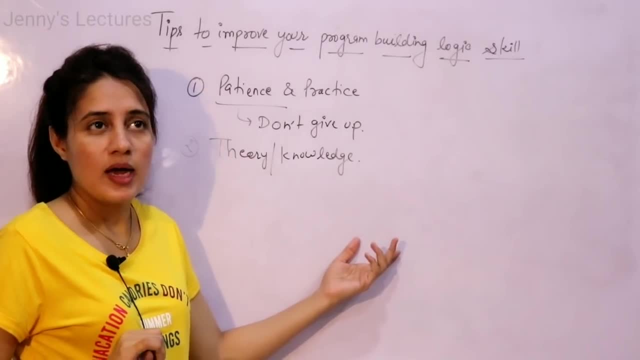 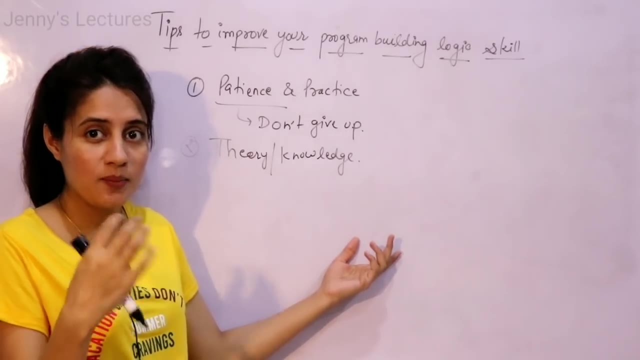 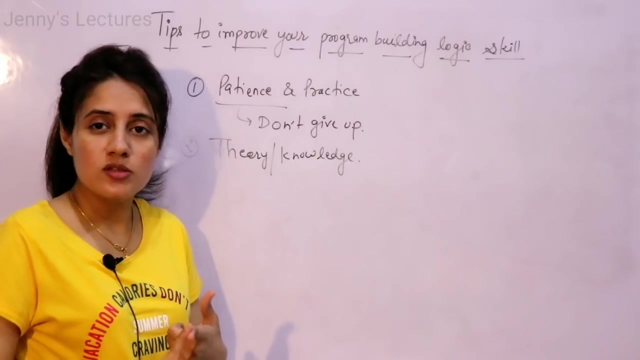 is very simple program. no need to write down this code, right? i will try some complex problems right? these kind of problems generally students do when they are beginners or when they are going to start. you know their graduation or something like this, right? so please don't do this. always try to write down, always go from basic to advanced. 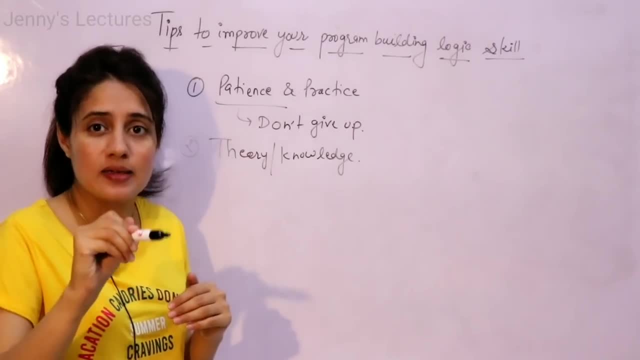 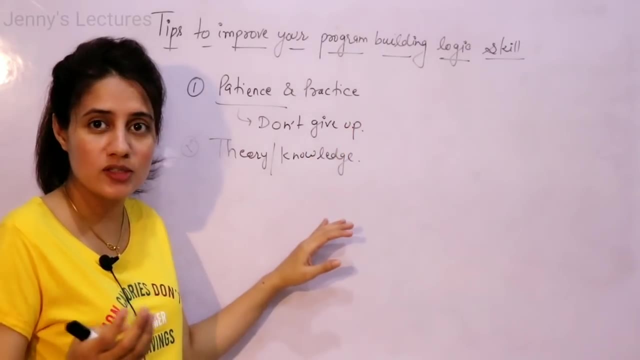 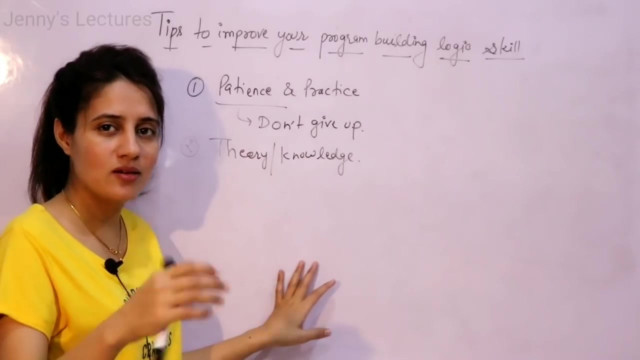 right and always to try to write down the code with your hand. right, because sometimes- see, it also happens with us in a maths you can say maths is also a subject when faculty is going to solve the problem on the board. you will think that it's very simple and definitely, if this comes, i'll 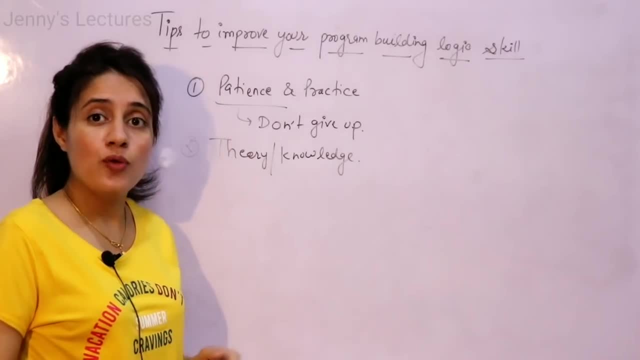 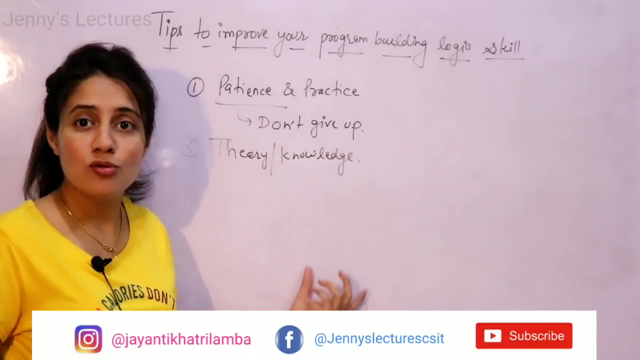 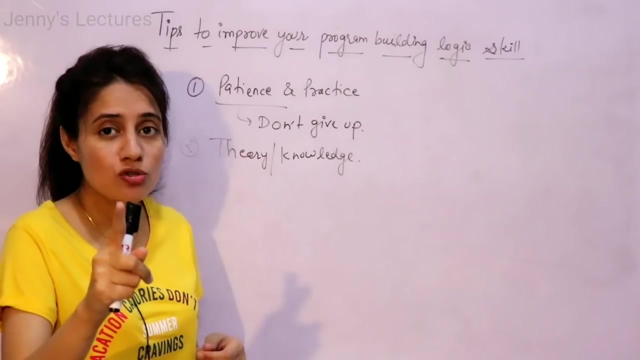 do an exam, i'll solve this problem in exam. but when it comes in exam, in that case even a simple problem is there, but you are not able to solve that problem. why so? because you haven't practiced that problem with your hand. this is also very important, so always. 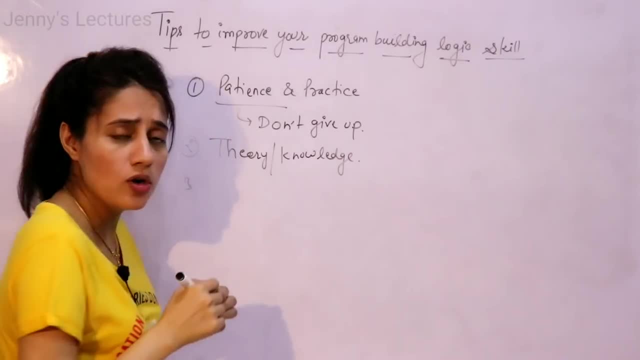 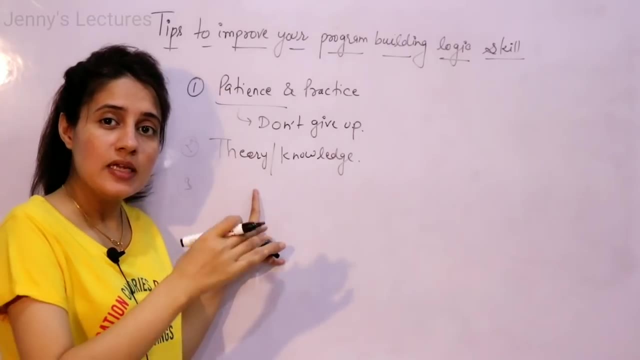 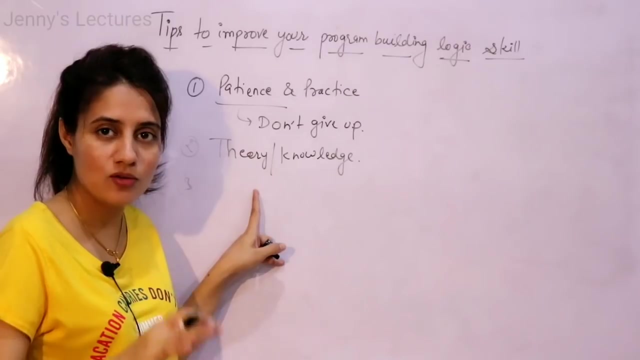 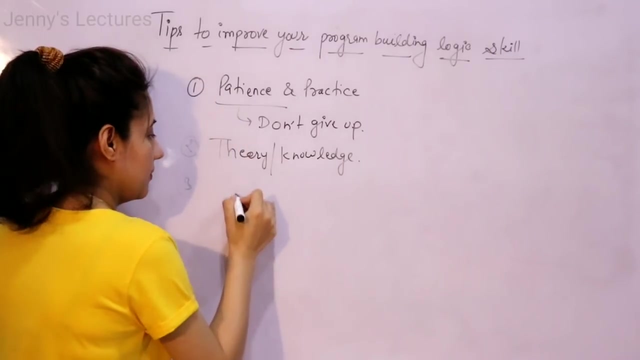 first of all what you have to do. third tip is what? use? pen and paper. this mistake also. generally students do what they'll do. they'll directly sit in front, in front of their laptop or computer, just use the id and type the code. it's fine. but it is better to use first of all pen and paper. this is very important and 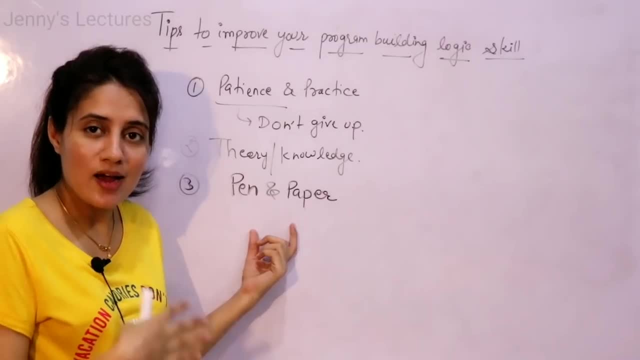 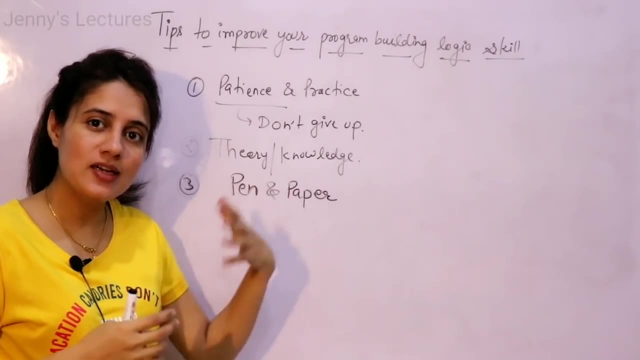 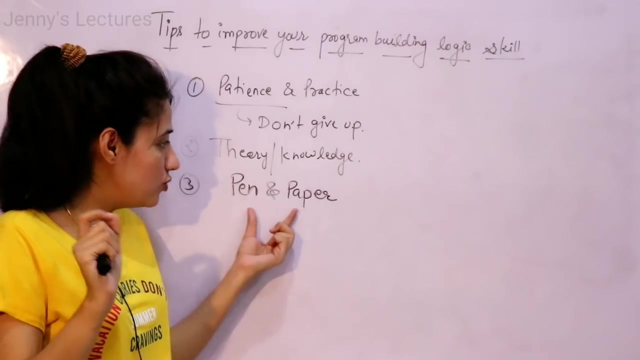 this is see these are. i have tried on myself these tips because obviously i was one of you when i was in btech. i usually done these kind of mistakes and these problems. i have tried and i have seen the improvement. that is why i am telling you: always use pen and 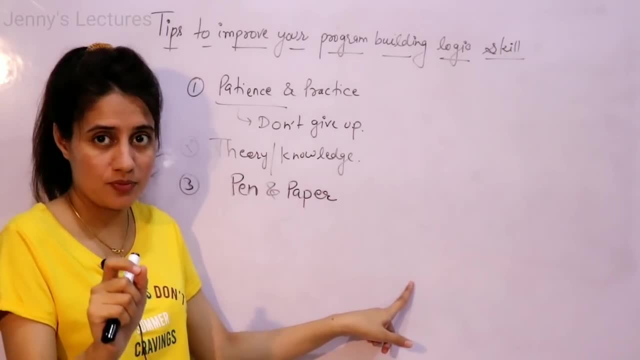 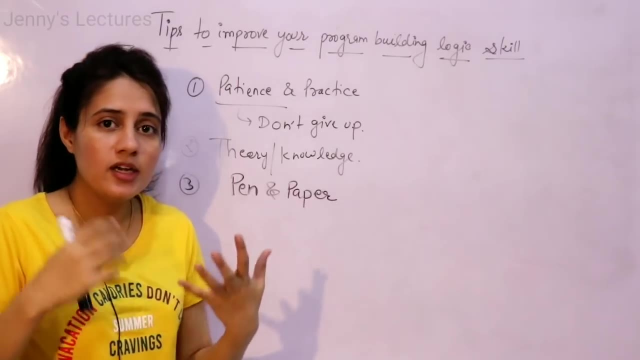 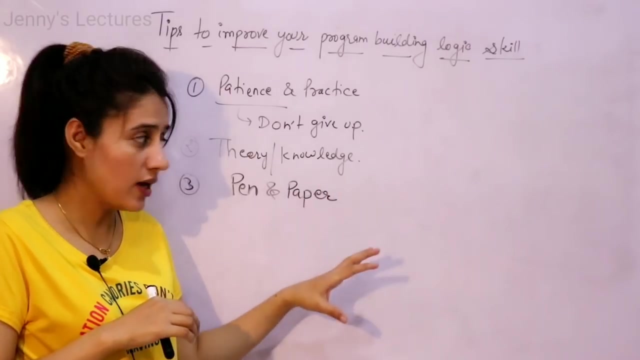 paper first of all. write down the code on paper first because see, obviously, when you will in, when you are going for a placement, in that case also the interviewer sometimes will ask to write down the logic right, and you haven't practiced for that. or you can say for any program writing on your paper, you directly. 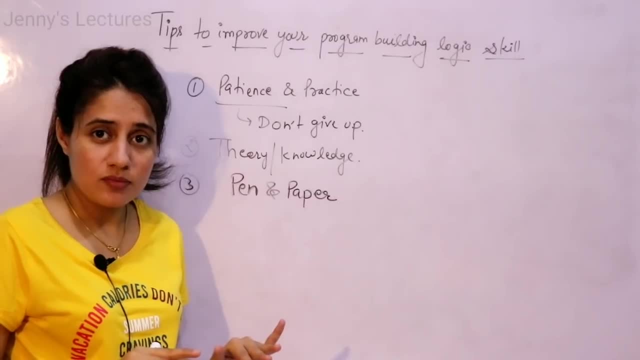 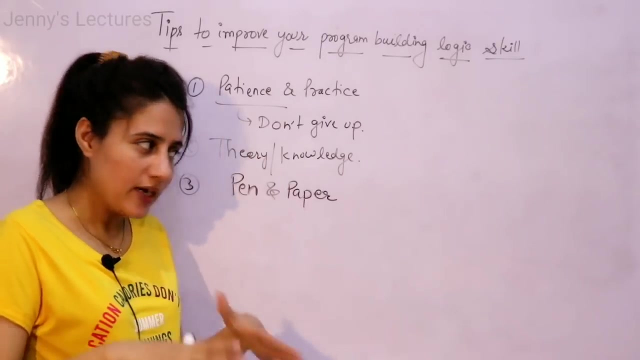 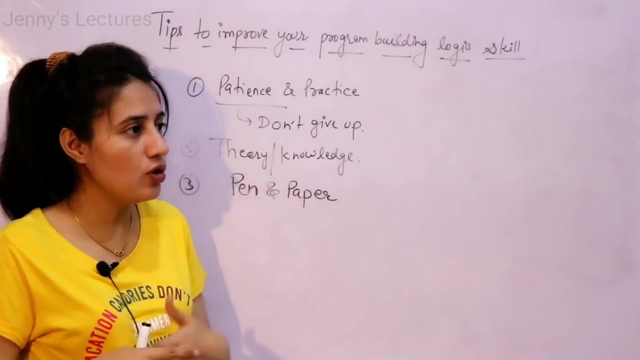 write down the code on that ide, right? so in that case also you will face some difficulties. even you know the logic. but writing on ide on laptop, writing on pen and you know, on a paper is different thing. so practice this thing also. first of all, right, always write down your code on paper if you are. 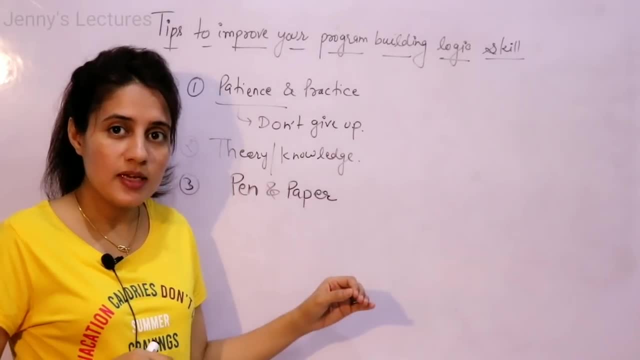 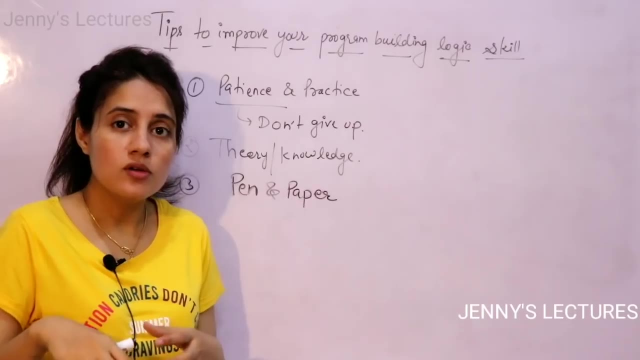 not able to think the logic, okay, fine if a problem is there, like suppose, if you want to check out a number is even or not even or odd. so first of all, don't just think that you have to write down a program. right, that is what the fear in. 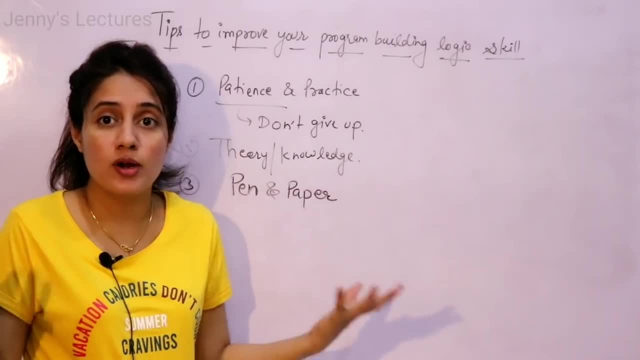 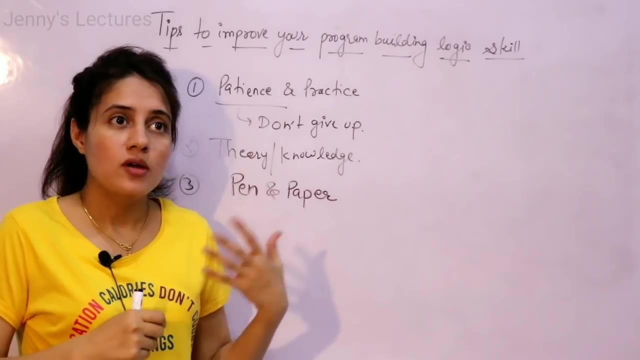 your mind a program. how will I write a program? I am NOT good, right? this is the same fear like when you go for any trip or when you go abroad, or when you go outside from your city first time. then you have that fear that how will I go? 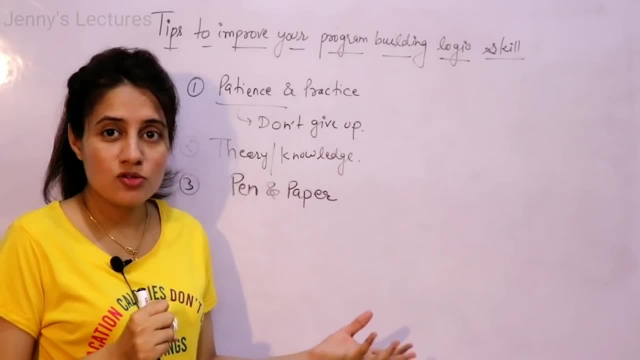 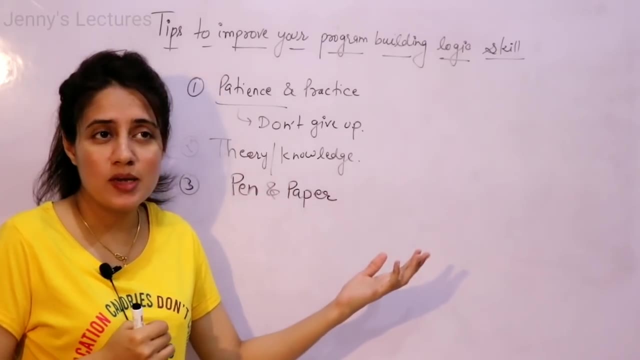 from where I should, you know, board a bus or where I will stay, and many kind of how I will. you know, I don't know about that place, how I am going to explore that place. many kind of questions, many kind of things are going in your mind at that. 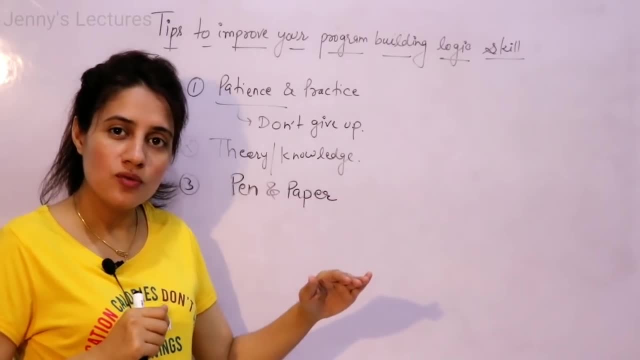 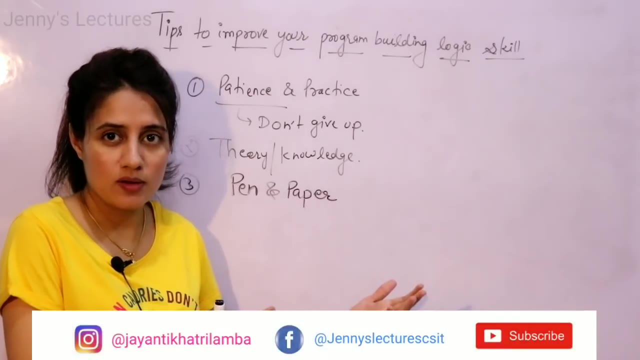 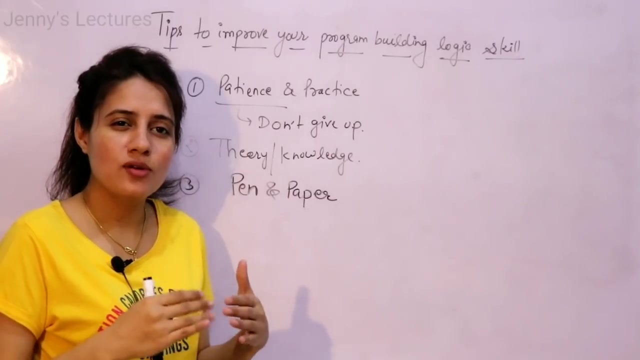 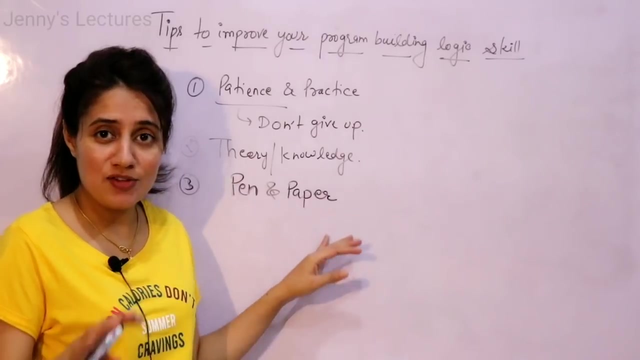 time right that fear. but once you go there you know automatically the teaching about me up with each other. and when you go second time or third time for a trip, at that time you will feel that you have less fear in your mind, like how will I go, where will I stay, and these kind of questions right same with 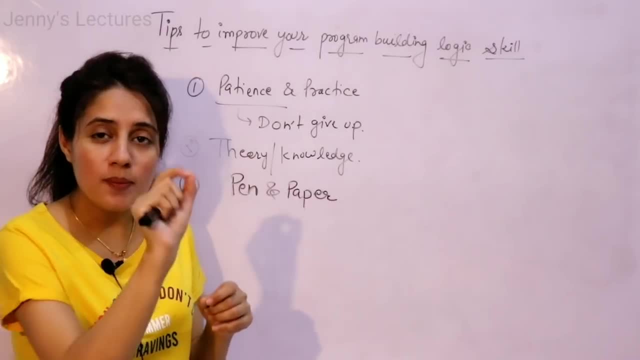 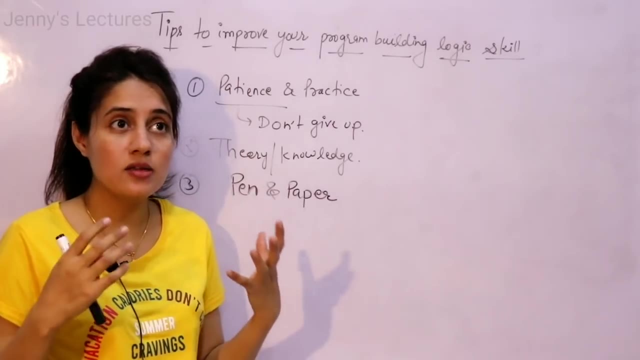 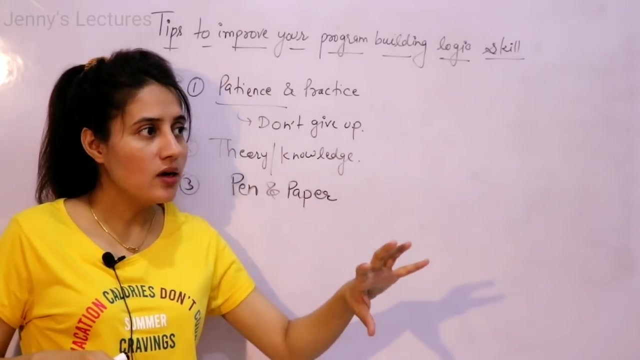 programming. you won't keep practicing till the you don't write yourself. till then in your mind it will remain: I can not do the programming and that has a fear. a program in your mind, right? so don't think that you have to write a program, just think how can I solve this? 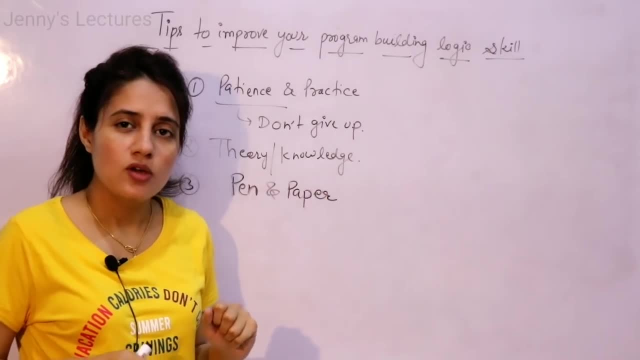 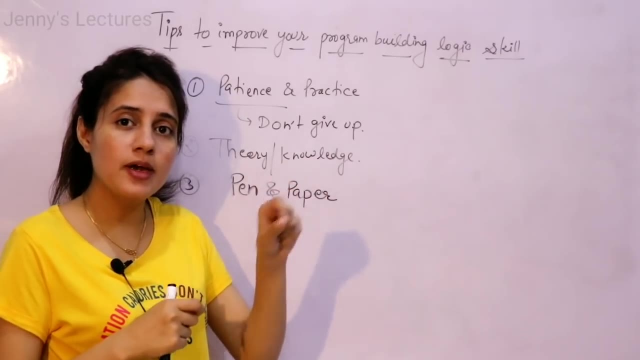 problem like how can I check the number is even or odd? for that what you have to do, just you can think in a mathematical form, right, if a number, if you divide a number by two and remainder of z is void, and if a number is a problem, say for G and thanks. 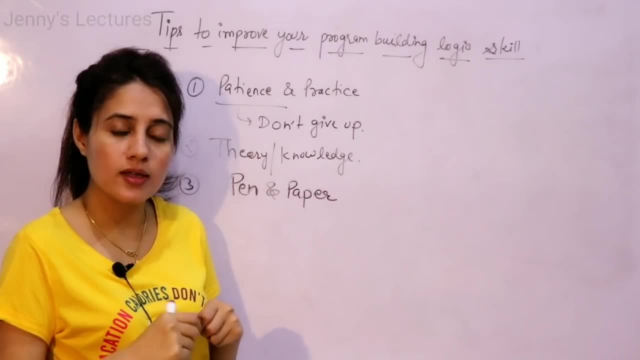 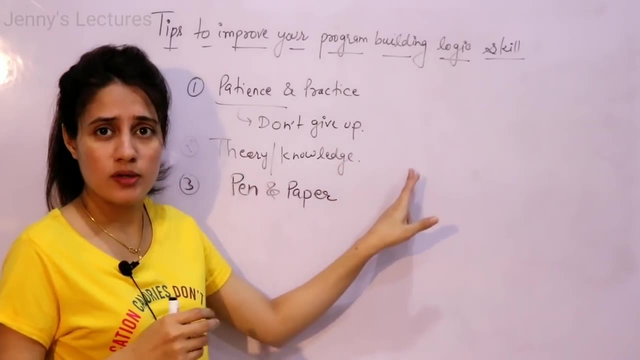 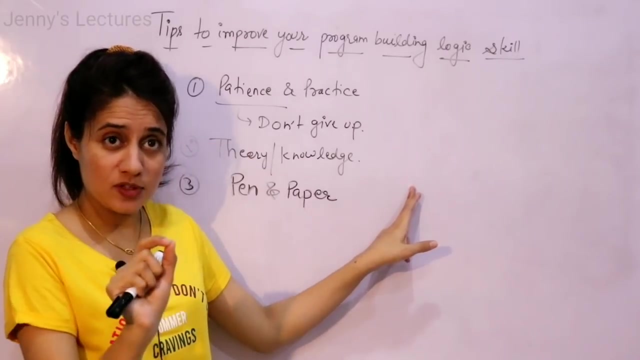 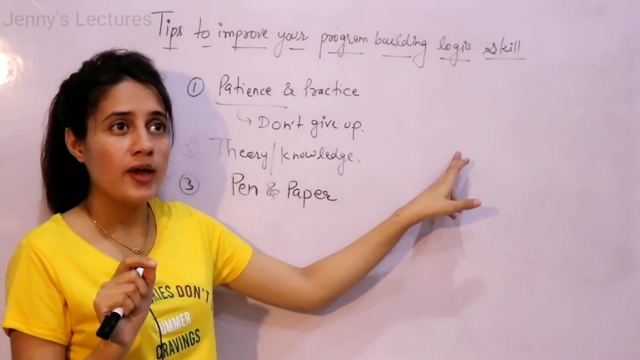 so much, okay, forÉ, that is even number. otherwise it is odd number, right? so for that, what you will do? you just write down either in hindi or english, in whatever language you are, comfortable program. just we need to take two numbers. if number divide by two and remainder is zero, then even number. 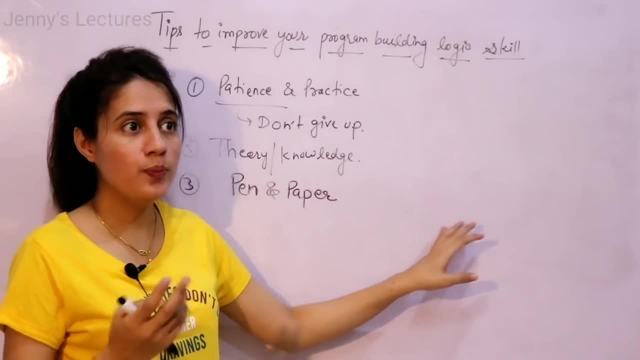 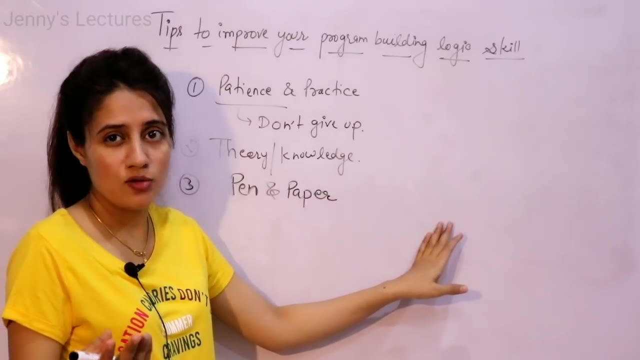 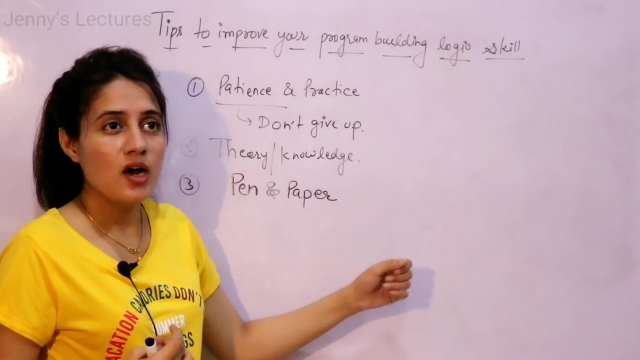 otherwise odd number. then we have to print also the result. right now, think how you can write down this. obviously you have the knowledge of at least any one language like c or c plus plus basic knowledge, the syntax. right then think how can i write down how can i take two numbers in c? 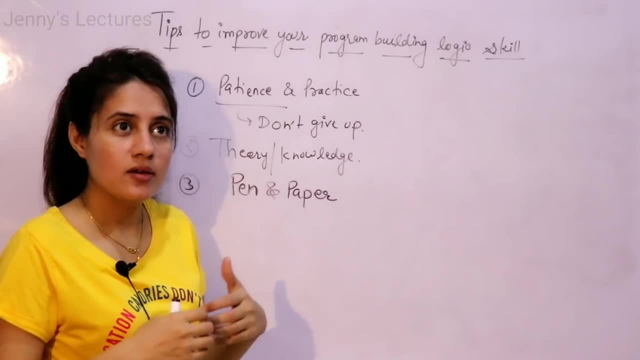 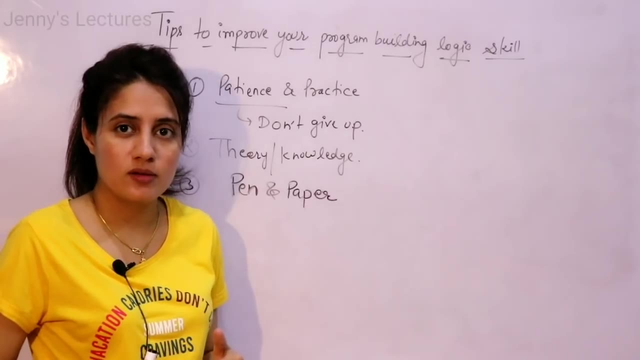 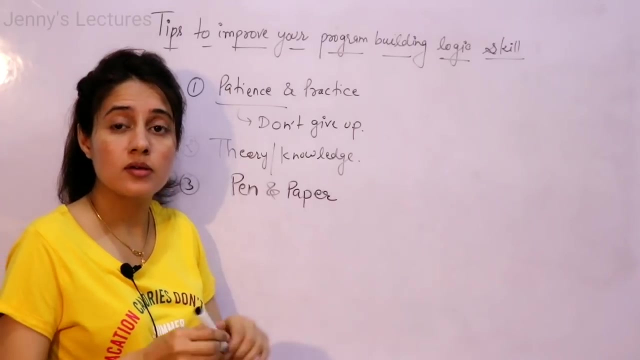 like int a or b. how can i write down the? you know if condition. obviously you know the simple syntax. then try to print the result right now. think how you can write down this. obviously you have the that in this form, right. and after writing the code on pen and paper, the most important thing is: 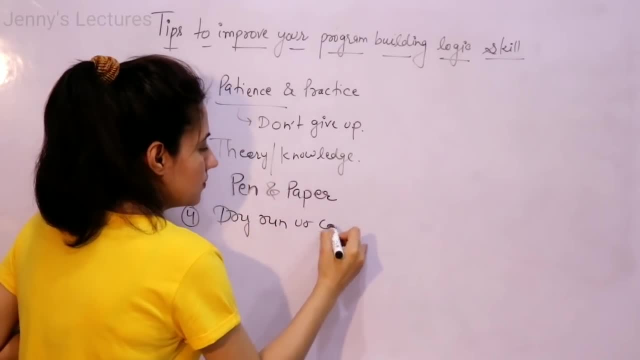 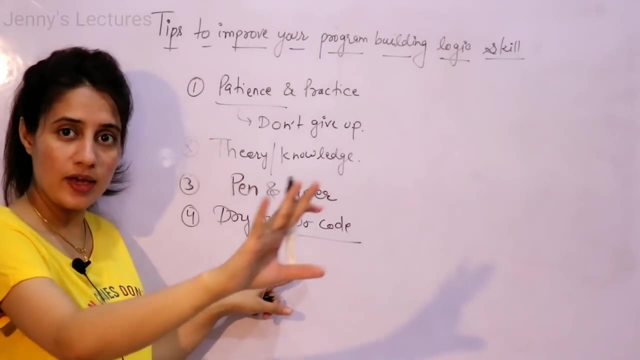 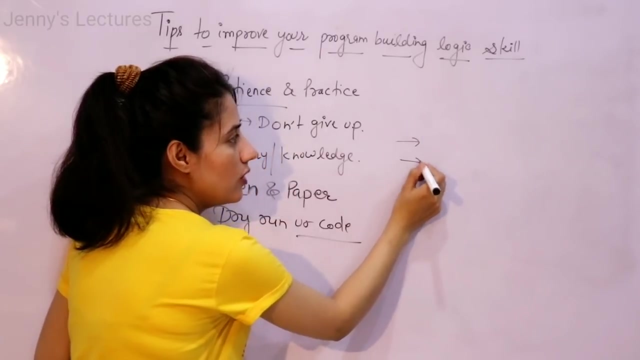 dry run your code. this is also very important. dry run means without using any compiler or any laptop or anything. you have to write down on a pen and paper and try to execute with your hand that first of all, you have to write down a code in this form right, and after writing the code on: 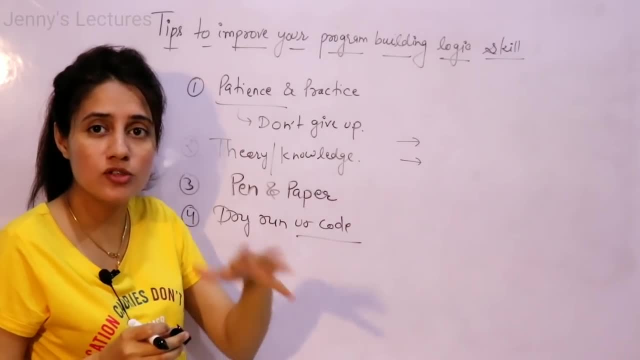 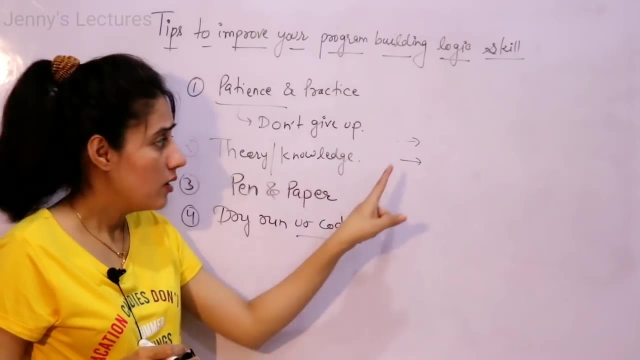 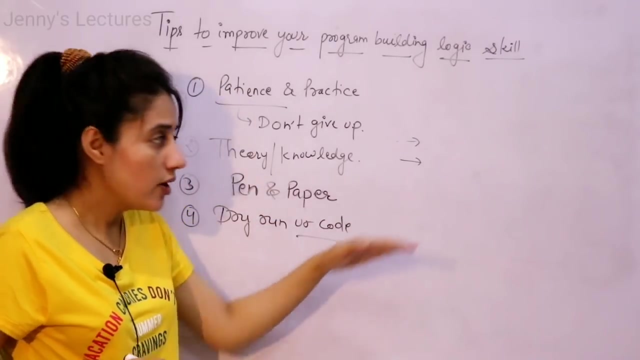 compiler will go to this line. we everybody know, first of all compiler we go will go to the main function after main function. this line is there. this will be executed. after that, this line would be executed. now, if this line would be executed, then what should be the output? right? so this is how try to dry run your code. this is also very, very, very. 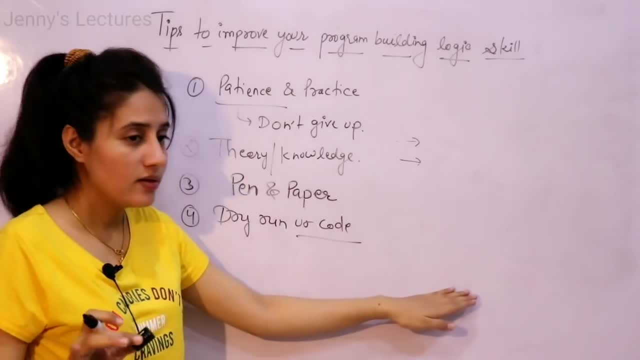 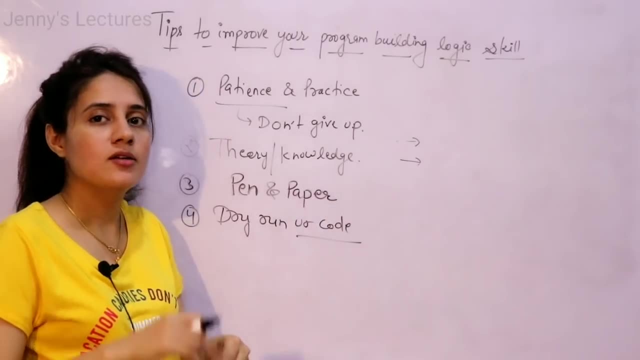 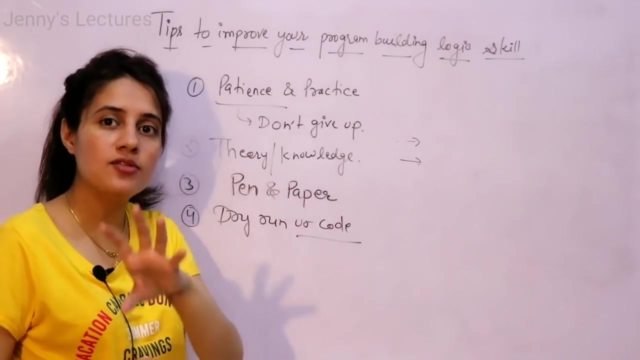 important tip right and see that what should. what will be the result after the compilation, after the dry run of the program. after that, just go to your laptop, use any ide, try to type the your code and compile and run there fine, and there also you can use the debugger. 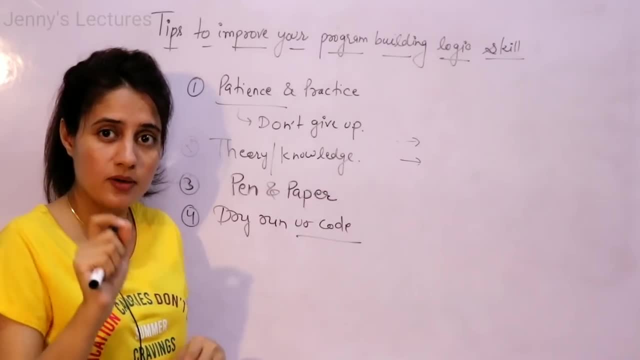 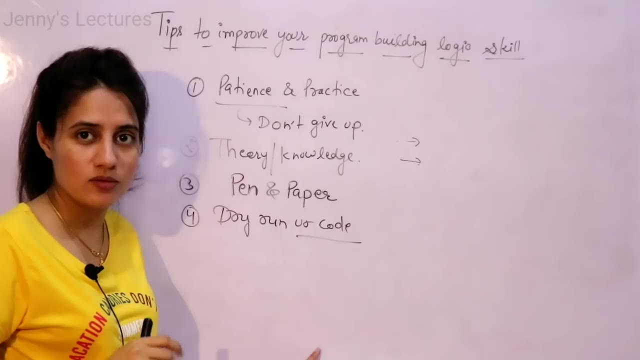 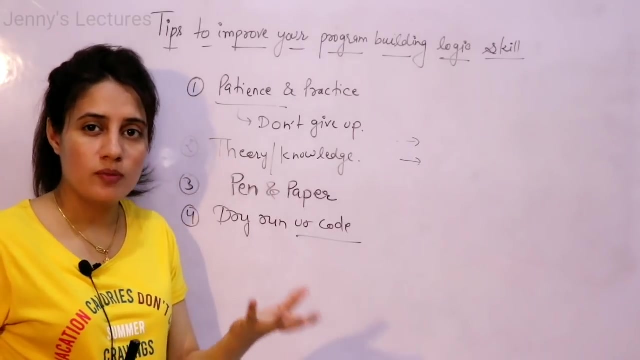 also, i hope everybody know how to use that debugger means step by step, how you can see that your program which line is executing now. which line is executing now, right. the compiler or the control is on which line, right? if don't know, then obviously you should use the debugger right, and then you can use the debugger on your laptop as well, so that 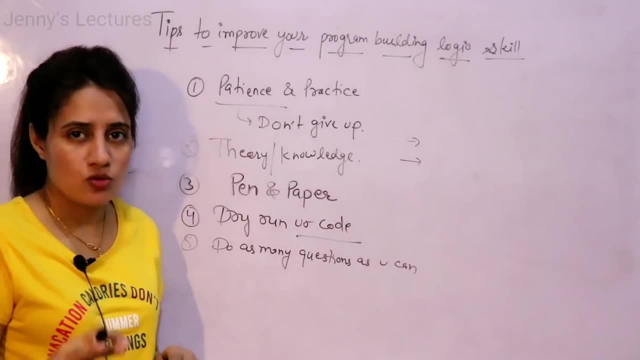 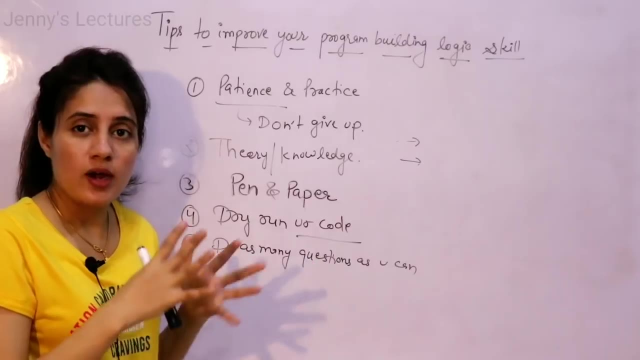 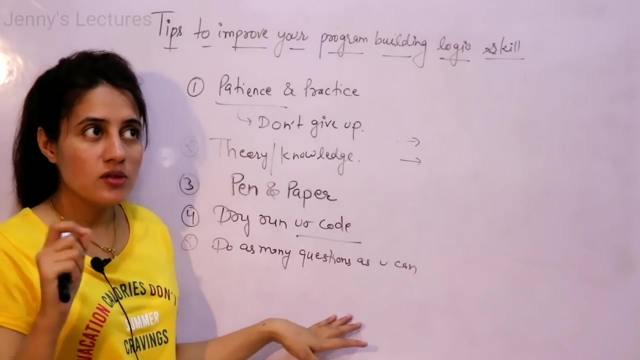 is what we are looking for. so the next thing is: do as many questions as you can right, like after completing one chapter. try to, you know, solve the problems based on that chapter. practice many problems right and see, it's not like that if you are stuck somewhere, if you are, 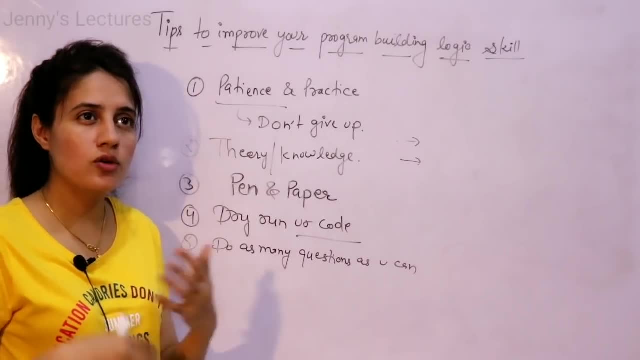 stuck on one problem and you are trying, you are trying, you are trying, you are still stuck. fine, fine, you can leave that problem. you just take a break after that, after 10-15 minutes, you can try that problem still. if you are not getting, you can leave that problem and you. 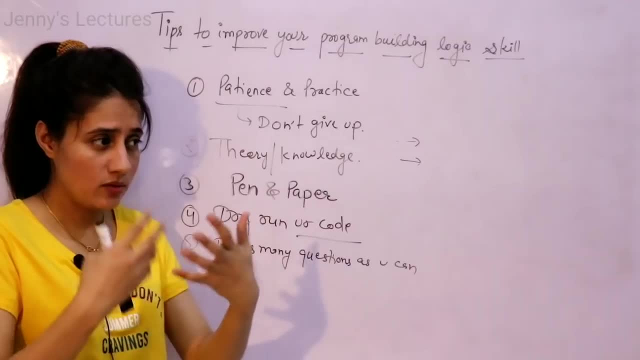 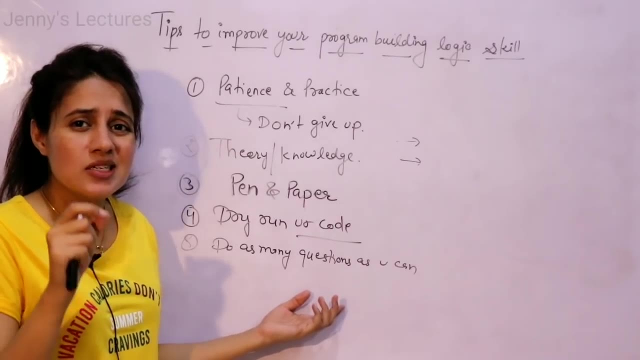 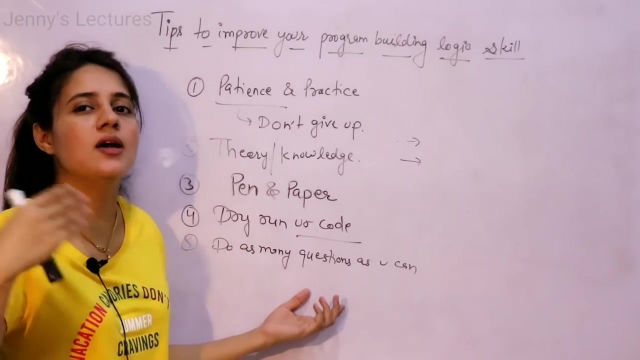 can move on. you can try another problem. maybe after completing 5 or 10- another type of problem- you will get the solution of that problem also. so do not just stick to one problem. if you are not getting, leave it, it's fine. there are many more problems, you can practice many. 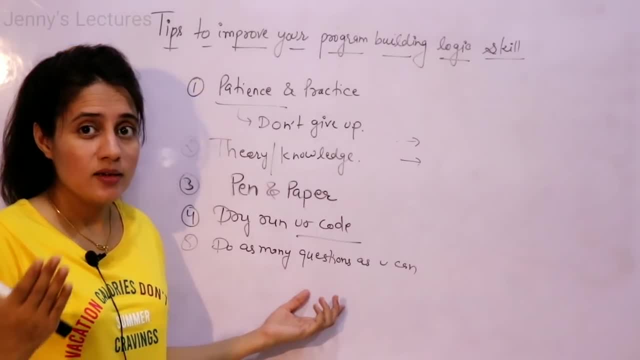 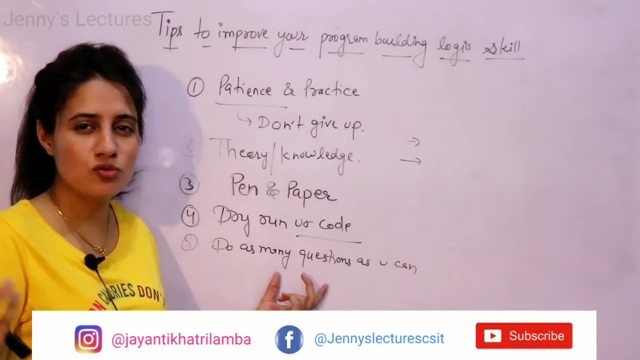 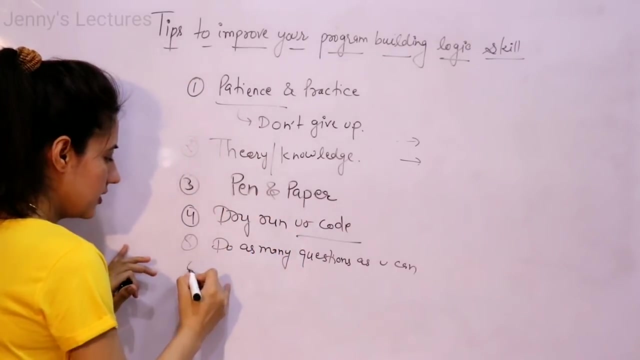 other problems also right. but don't get demoralized that I'm not able to solve this problem. it's fine, it happens, right. it's not like that. everybody is able to solve every type of problem, fine. next thing, which is very important in this, in this case, is regularity. you must be regular. 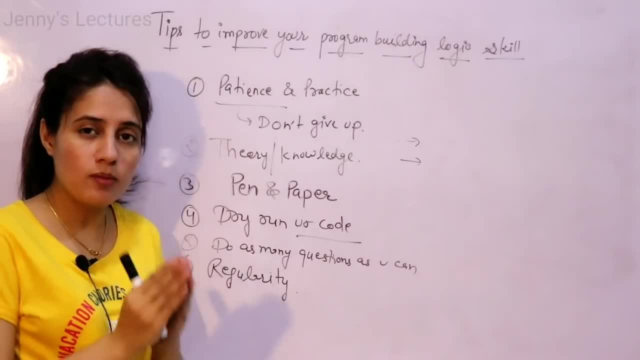 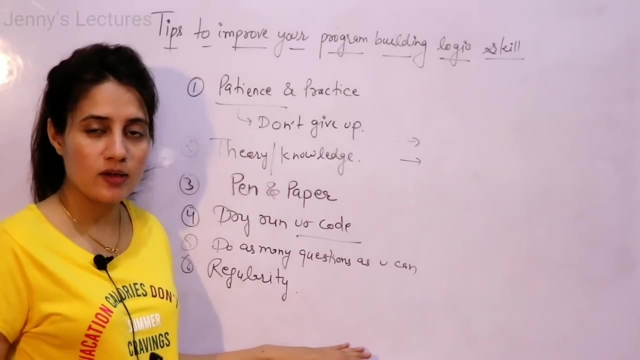 right if you are solving like 15 problems per day. so you must be regular. it's not like that you are getting the solution. but it's fine, right, that's a minute you can get. the suppose you are solving 10 problems in one day and one day you will do that i'll solve 50 problems. 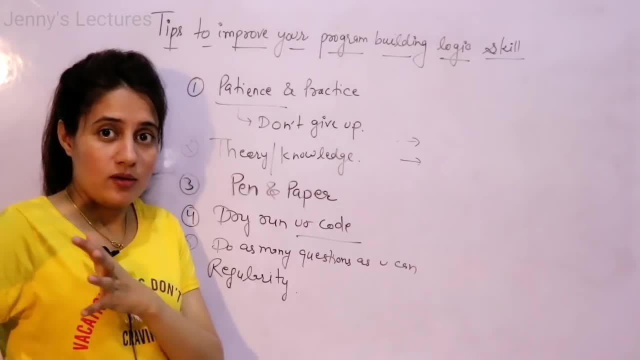 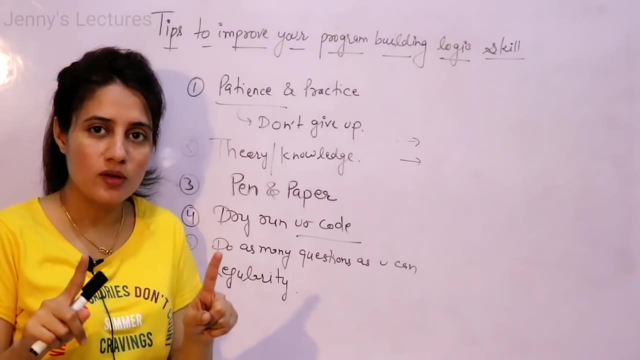 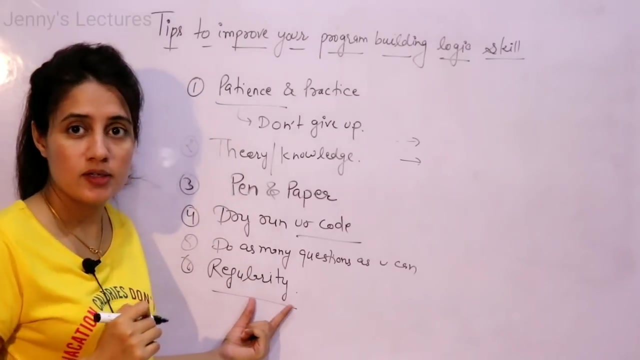 one day and then we'll get. we'll be, you know, uh, not, we'll be not solving problem for five days and after that another sixth day i'll solve 50 problems more, no, solve 10 problems, but daily, on daily basis. this is also very important. see, these are very simple. you know tips and you will feel. 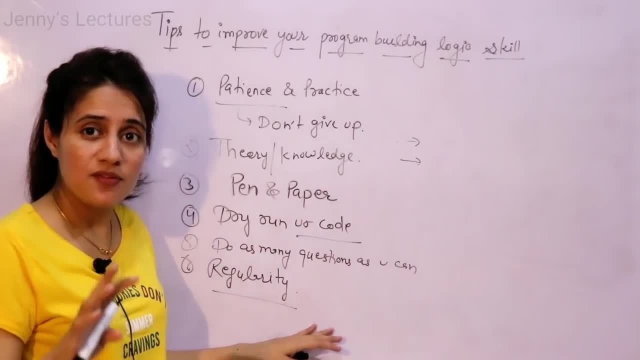 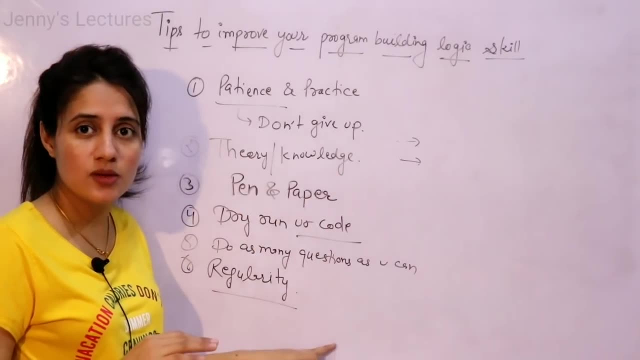 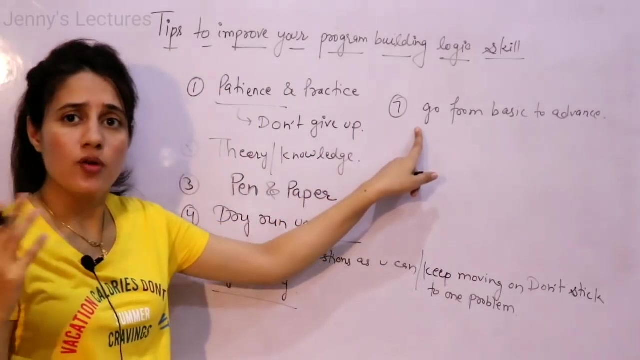 that these are of no use, but definitely these are going to help you. after 15 days, or maximum after 30 days, if you are going to follow these tips, definitely, definitely, i guarantee you, you will feel the difference and always go from basic to advance. it's not like that. these are basic. 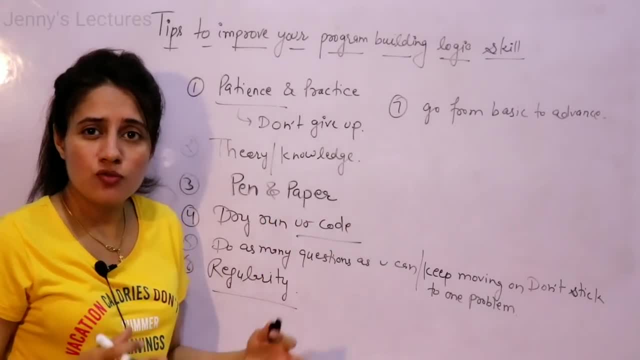 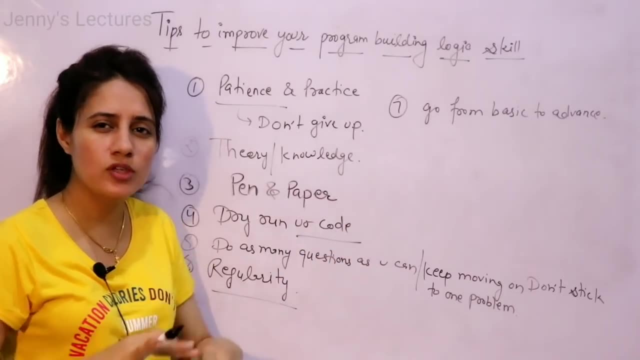 things like, uh, addition of two numbers, subtraction of two numbers, maybe finding even node, and you will feel that these are very simple. no need to write down these kind of problems. no need to all these kind of problems. i'll switch to complicated problems. this is the you know. 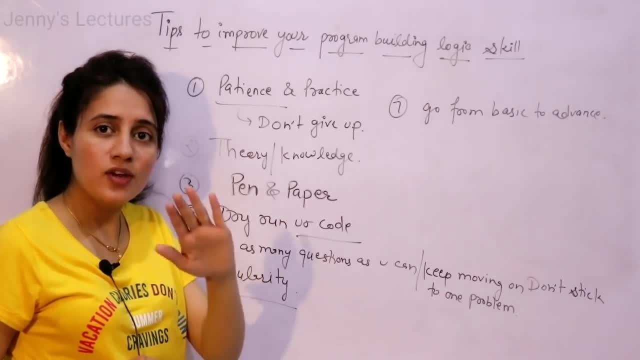 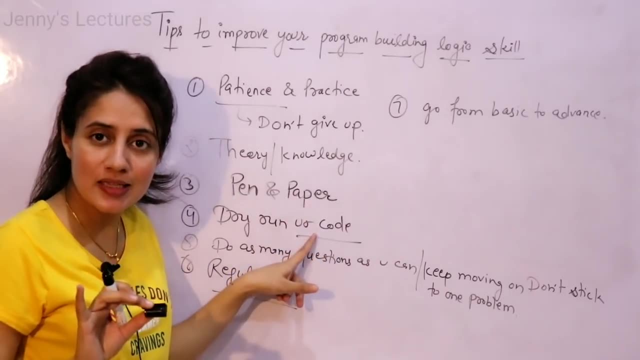 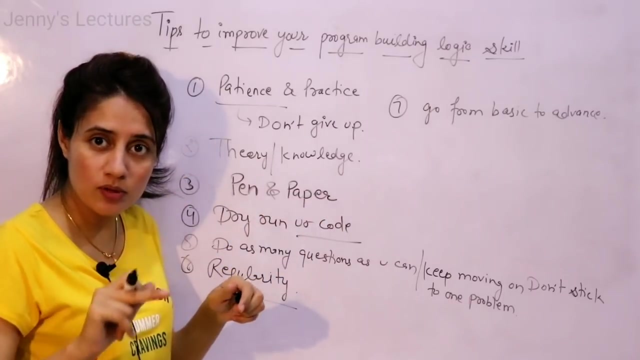 common mistake students do no. even if it's a problem of printing, hello world, you have to do it with pen and paper, first of all, dry. run that thing, after that on your compiler, even if it's addition of two numbers, use pen and paper. write down that problem if you are not able to write. 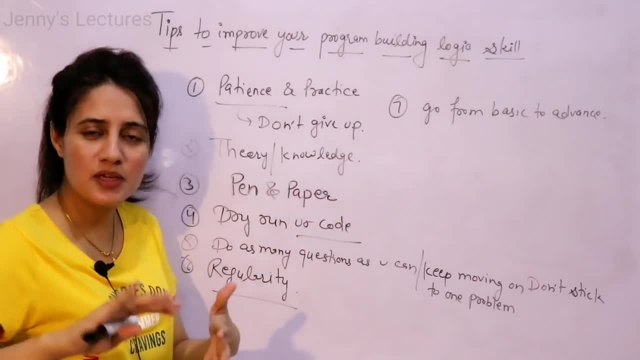 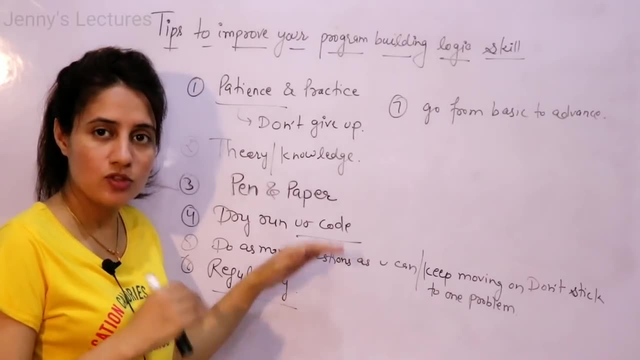 down the code first of all. obviously, you can write down in hindi or english in simple steps. what you need to do then: try to convert it into your programming language, syntax right, just do these things. after that, go to the advanced level right and try to solve as many problems as you can. 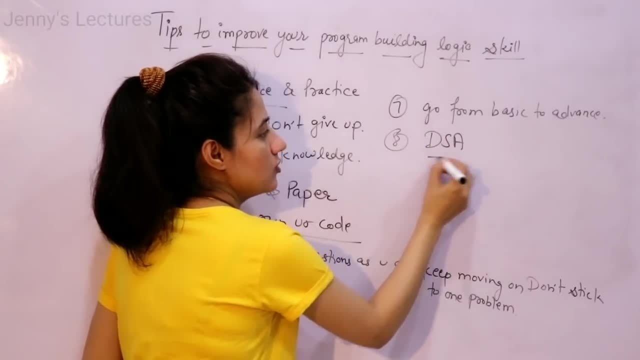 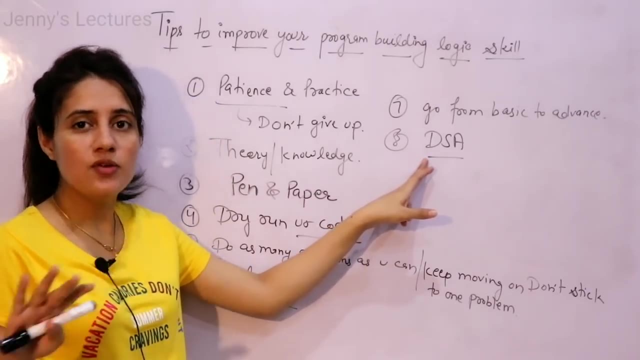 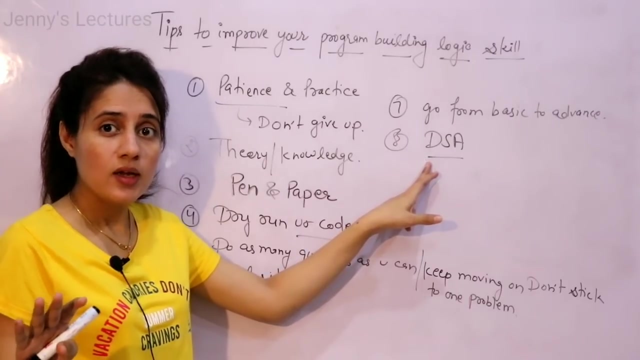 next thing is what? obviously here, dsa concepts are very important. right, learn data structure and algorithm concepts. i have already uploaded many videos on dsa concepts. i think it's around one, one, two videos. you can go through those videos, right? and i have also applied these kind of techniques. i have properly write down the code. 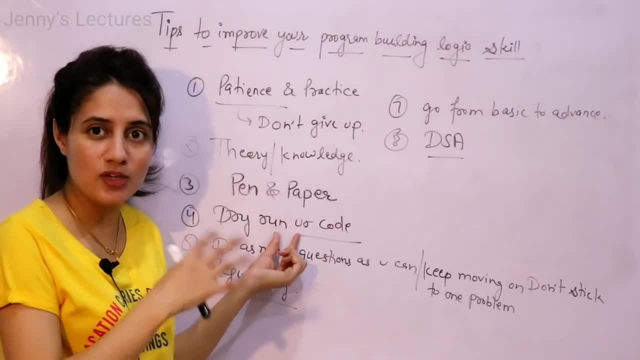 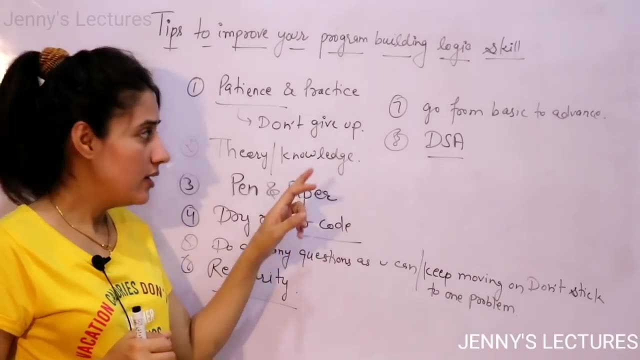 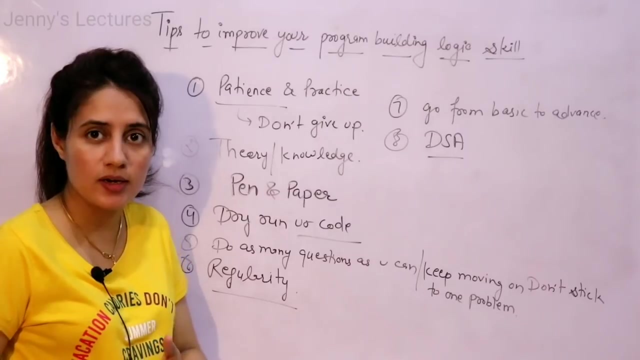 on the board and i have dry run that code in the video. right, so go for the dsa concepts like you are. first of all going for the array read. take the theoretical knowledge of that concept. try to solve the problems on array 1d, array 2d, array, multi-dimensional array, right, first of all, 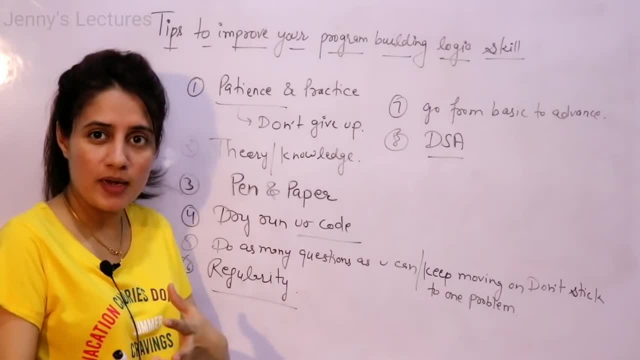 simple operations on that, like how to insert, how to delete from array, like this, after that some complex type of operations- fine, but try to solve many problems on that. it's not like that. you will stick on the particular concept only, like array only. you have to keep moving on. 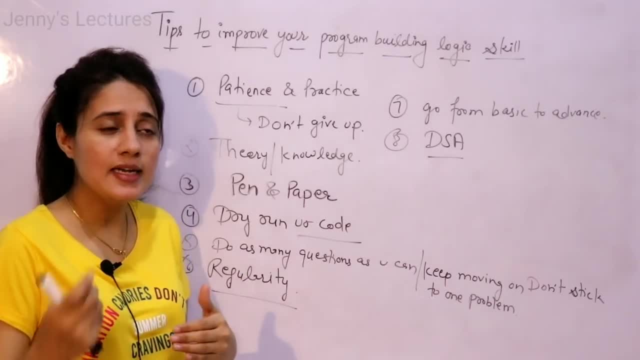 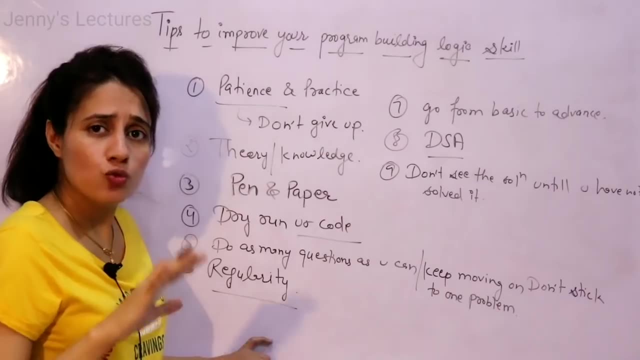 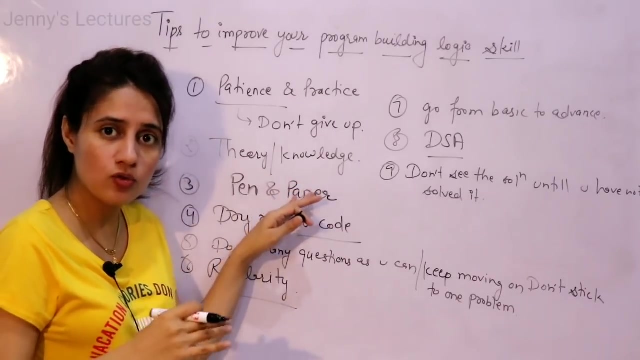 also face new problems every day. at least one new problem right next is: do not directly switch to the solution. first of all, try to solve it at your own. try to write down the code. try to dry run that code, bottom line right- never dry run that. or try to compile and write down on your laptop if you are stuck, then you can see the 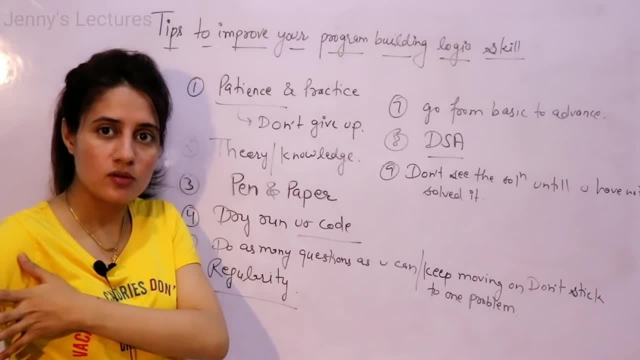 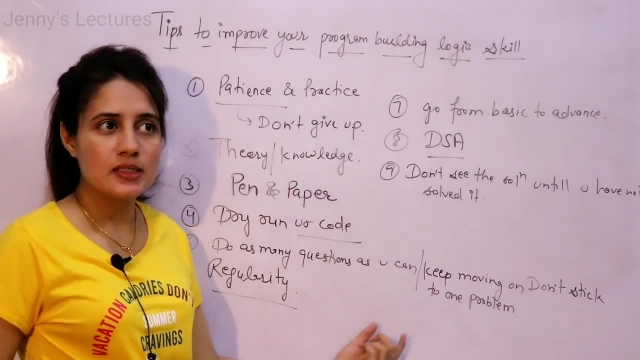 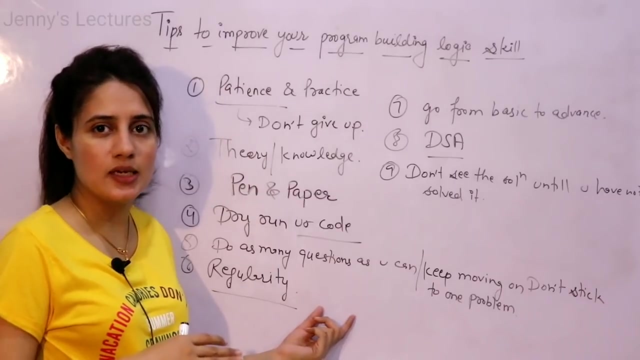 solution directly. don't jump to the solution. see, many students do what. there is a program, you have to write down a program. they'll directly see the solution and they'll try to understand. and yeah, obviously this is very easy. you can understand that thing very easily. but understanding of a 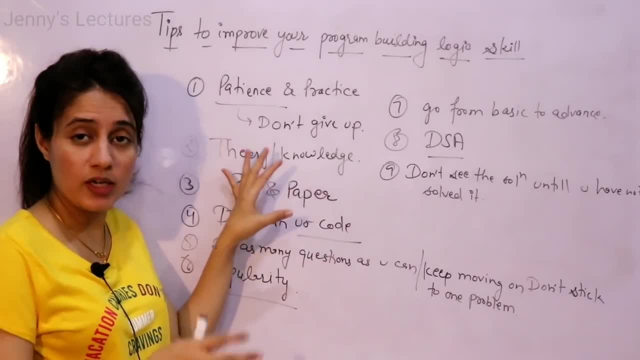 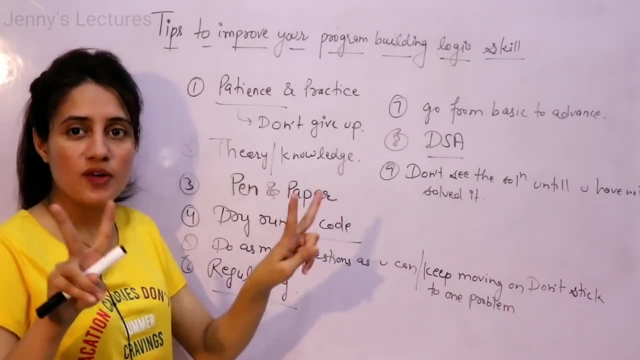 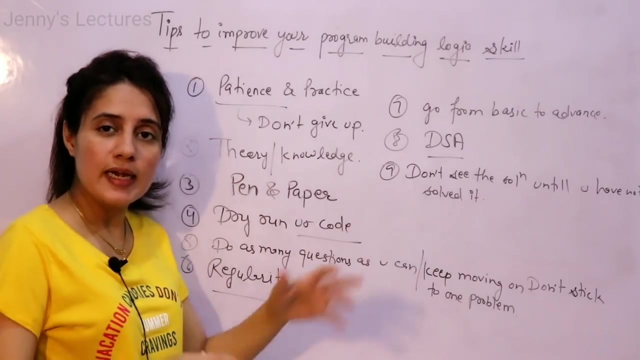 given program or given problem. you know, sorry, a given program is different than writing your own program, writing your own logic, right? these two are different thing. don't mix these two things, right? so please, first of all try to solve. if you are not getting it, then you can see the solution. 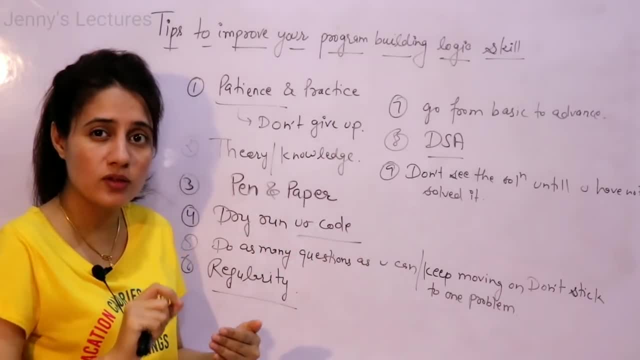 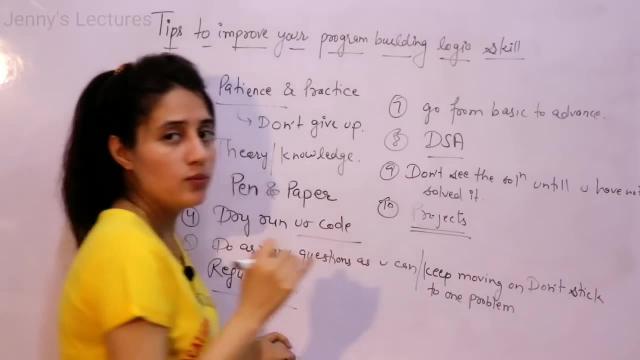 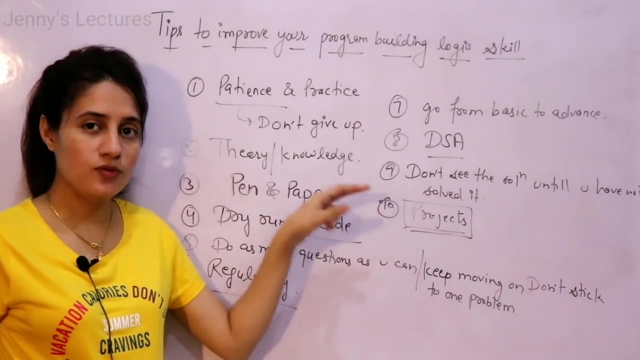 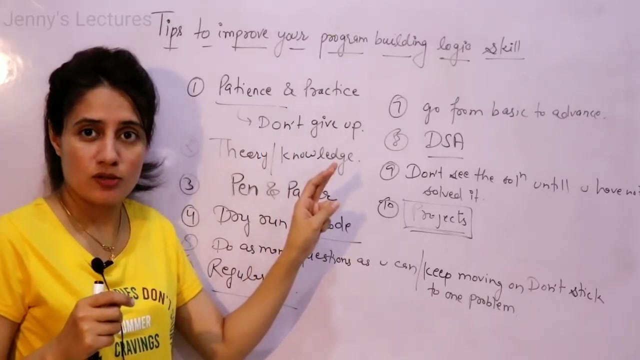 you can read the solution. try to find out where you have done the mistake again. try to solve another type of problem. fine, and here we are. the most important thing is projects. you have to work on projects if you know, you seriously want to feel that you have that capability, that you can build the logic. but after trying all these, 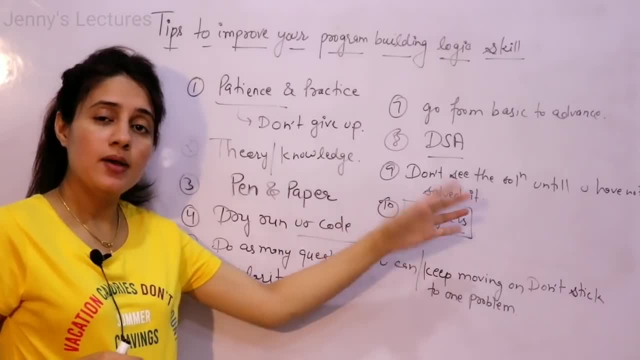 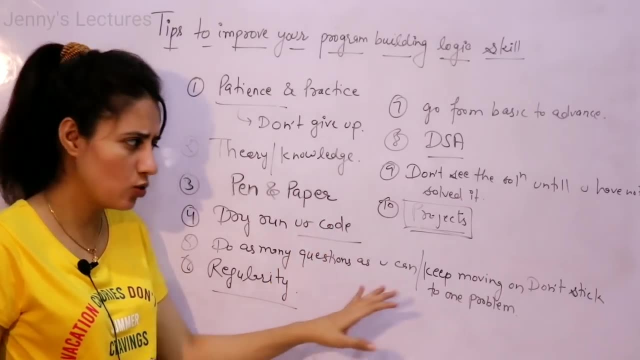 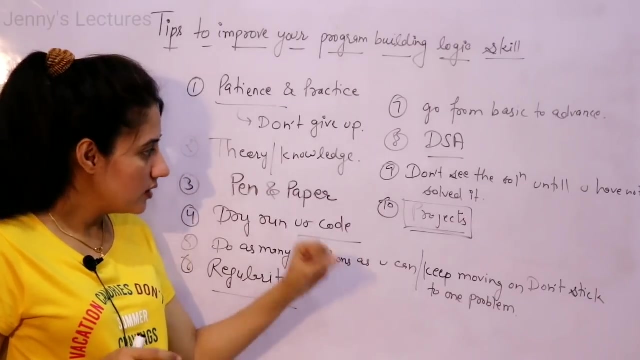 things. it's not like that. I'll directly make a project. so that would. that would be good. I'm not going to practice these kind of things. I'm not going to practice the questions or nothing like that. I'm directly willing to build a project. no, because sometimes what happens if you're in that? 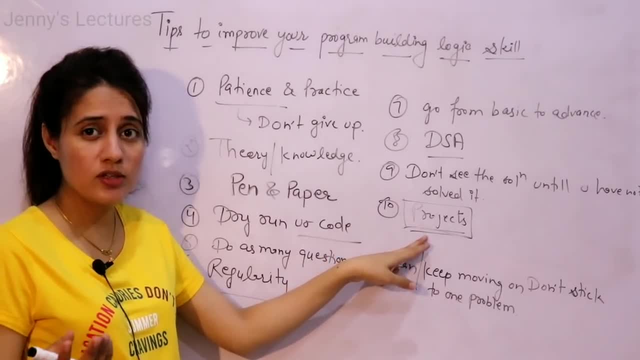 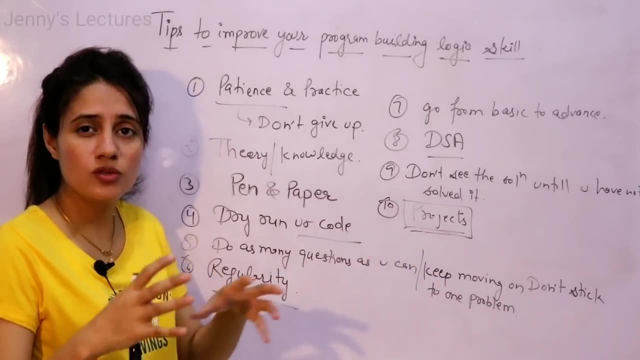 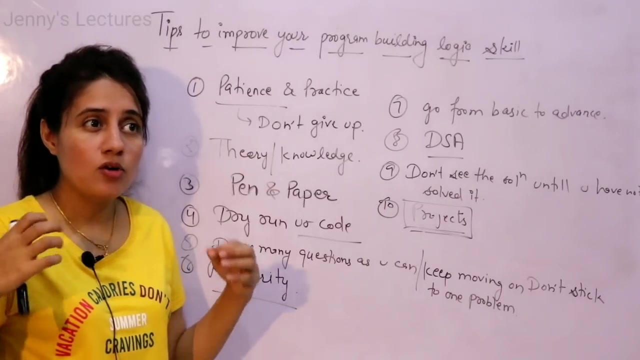 case you're not able to, you know, build that project, then you will get demoralized right and I'll see. I'll recommend that. first of all, try to go for simple projects. it's not like that. in, you know, first attempt, only I am going to make any complex type of project or complicated project. there is a database connectivity, also many buttons, also many kind of kind of things. so once you apply, there is database connectivity also, many buttons, also many kind of things. that first attempt. only I am going to make any complex type of project or complicated project. there is database connectivity. 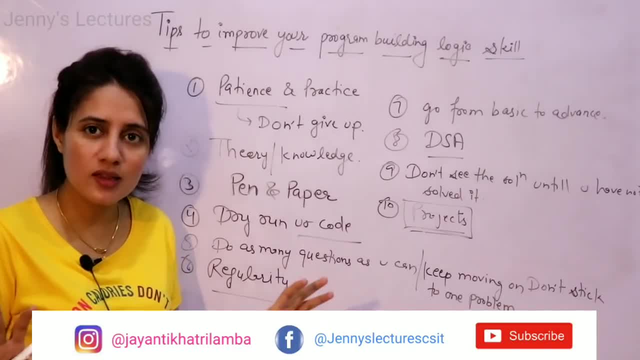 also many buttons, also many kind of things that are down the diynı technique, are the ones which customers will centre on and which project that's to be maintained, and even when you give that to them, many kind of things. no, don't think like this. first of all, you can take a simple project. 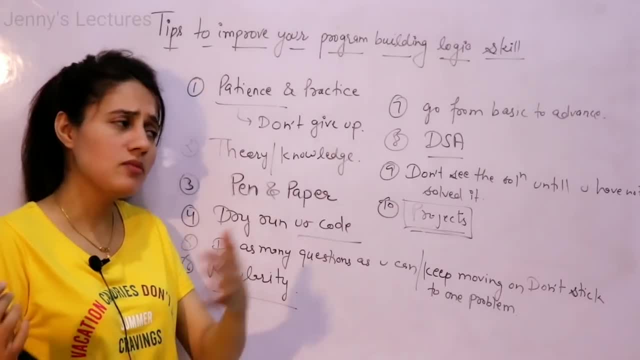 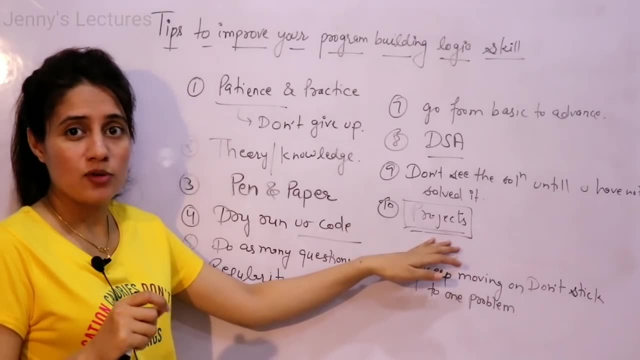 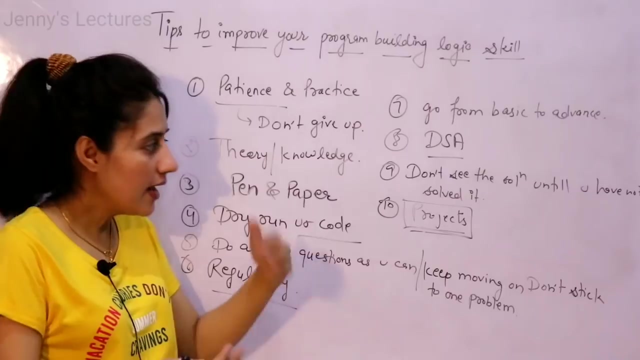 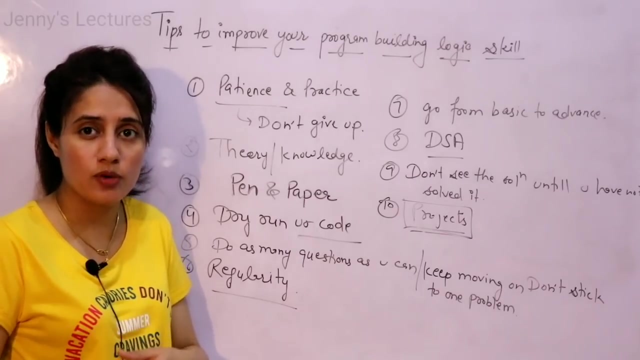 also without any database connectivity right. try to implement, try to build that project. in that case also, when you have built that project, that will boost up your confidence definitely. right after that you can enhance your project. after that you can, you know, learn how to connect, how to get the database connectivity in your project right. after that you can enhance. 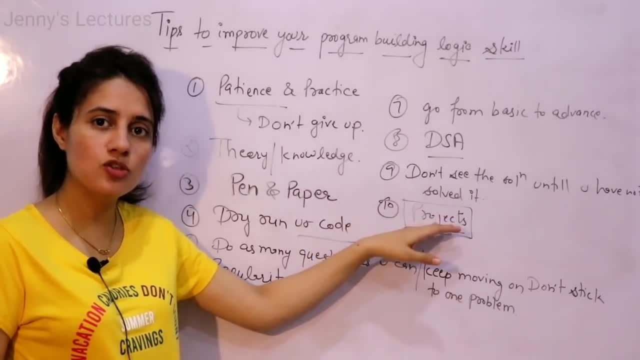 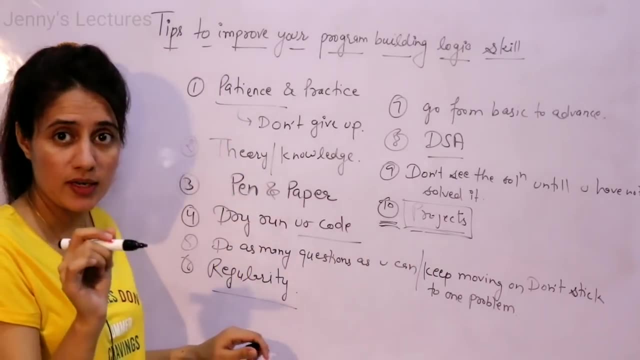 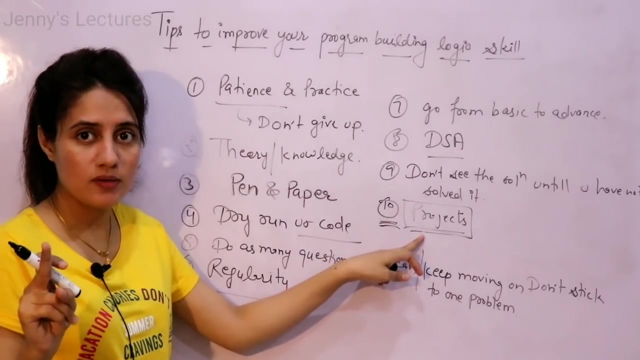 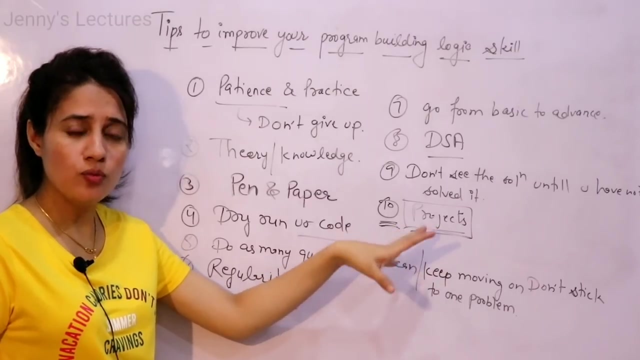 your project and you can embed that feature also, the database connectivity- in your project, right? so this is very important. on the point here that you have to work on projects to improve your logic building skills, this is very important, right, and suppose you have sincerely tried all the things. you have practiced many questions and now for 1 month or 2 months, 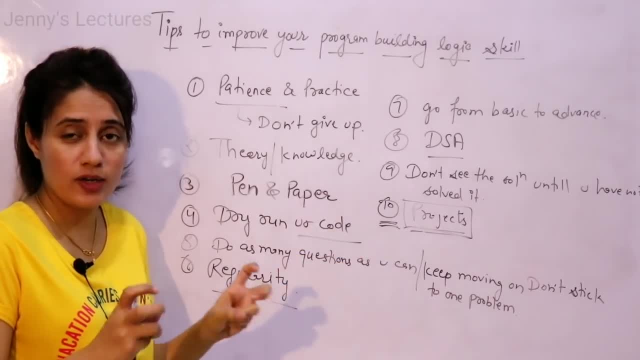 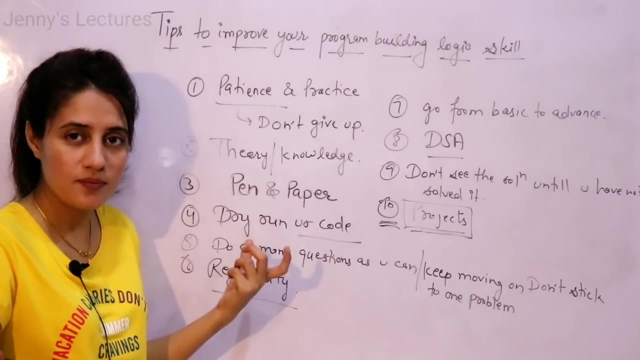 of time. you have already observed 2 colors or 2 harps for any of the scorcher in that, and now you think that you are able to think the logic you can able to. if you have given a program, you can able to think the logic of that program at least 50 percent, 60 percent, 70 percent, right. 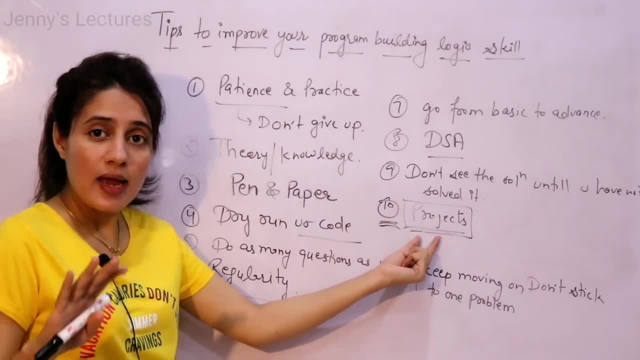 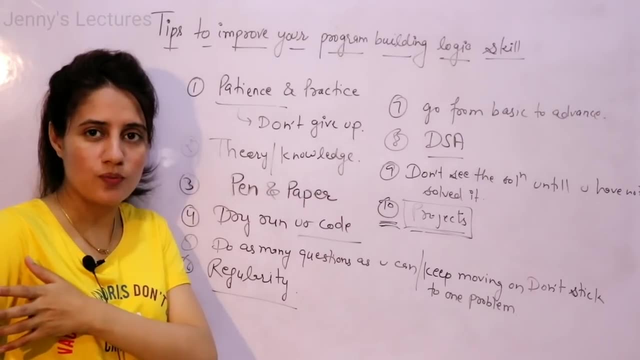 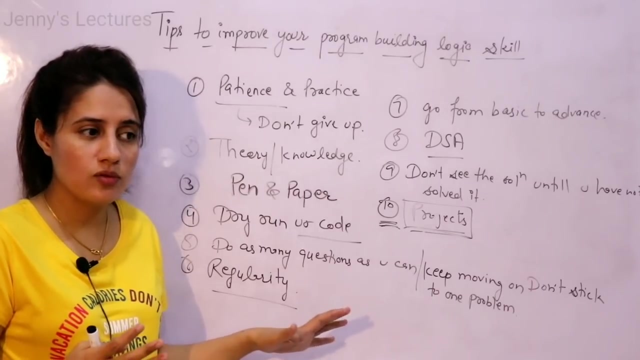 then you can go for the projects and while making the projects, at this time you can check the code of other people also. right, try to understand the code of other people. maybe you are writing the code, which is very complex, or their time complexity is high, or space complexity is high, maybe someone